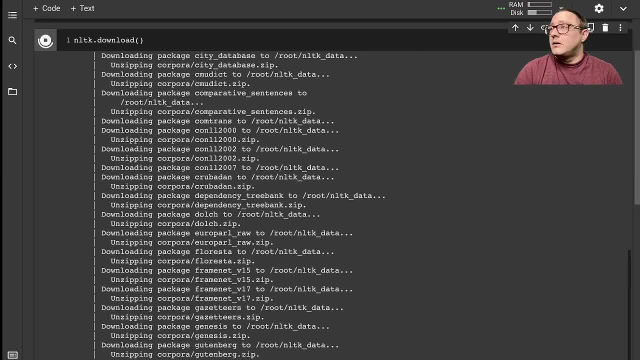 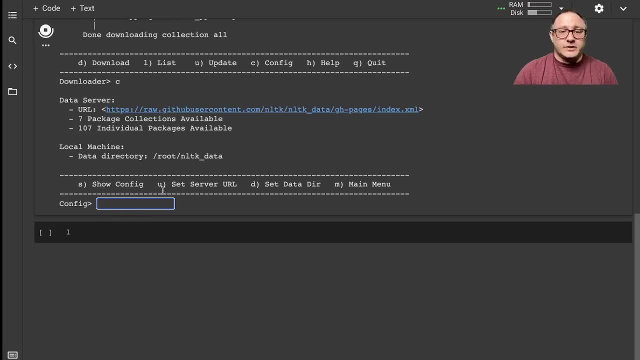 that we don't waste too much time. So once this is all done, you can actually go ahead and hit go through, and right now I'm in the configuration setup So we can actually take a look at the configurations if we want to. but I'm going to go back to the main menu and we're going to do Q for 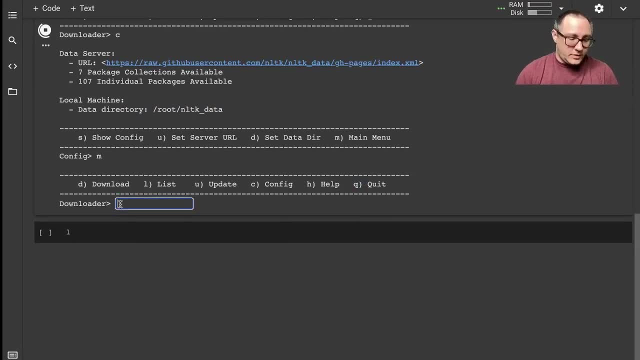 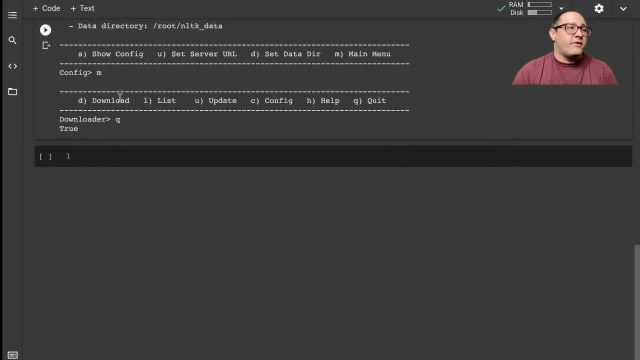 quit in here and, oops, Q for quit, And then that will break you out of the installation so that everything is good to go. So, as I said before, we're going to be using the SMS data set, Spam data set in here and let's go on and download the data. So we'll use curl and I'm going to put 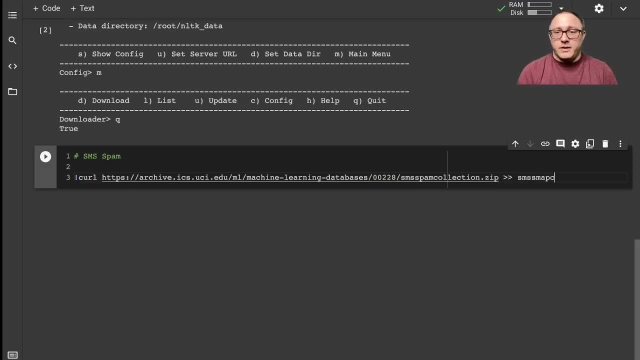 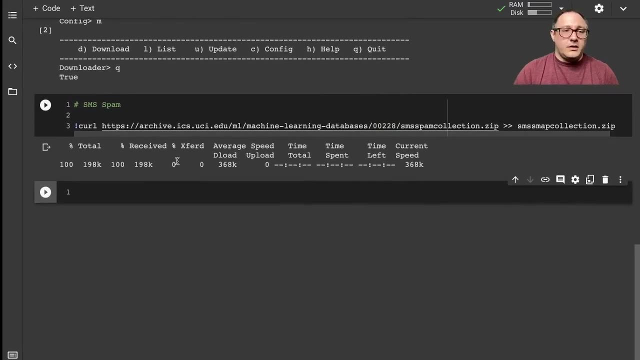 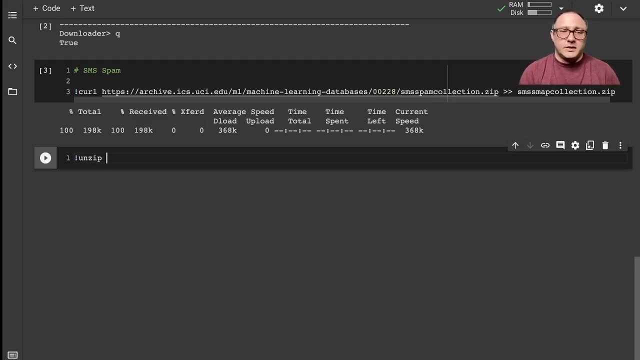 this into the SMS spam collection dot zip and we'll let that download really quickly. And then again, once it's done downloading, we want to unzip the data zip and I'm just going to unzip it. Let's see what do I want to actually do. 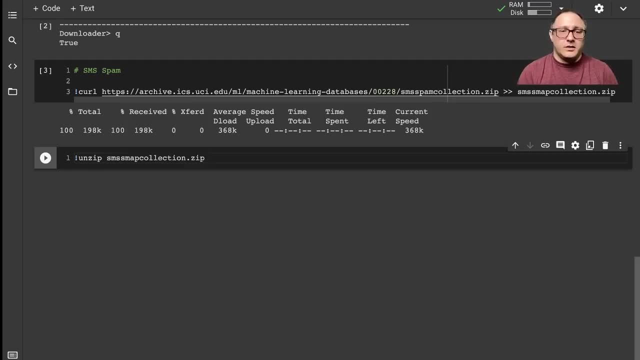 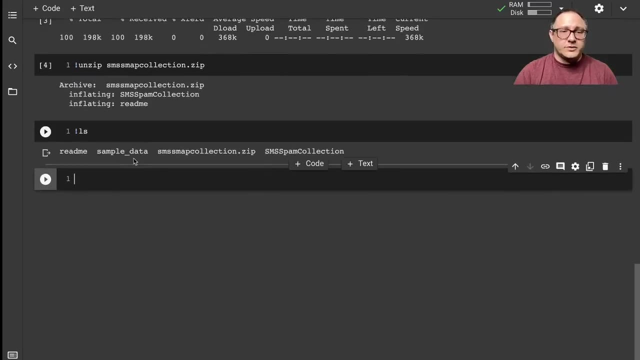 Let me put it here and, yeah, I'll just unzip everything here so we can take a look at what variables are. So they have. we have this sample data, which is a small subset of the data. We still have our zip, the readme file, but this is actually the collection that we want. Let's take 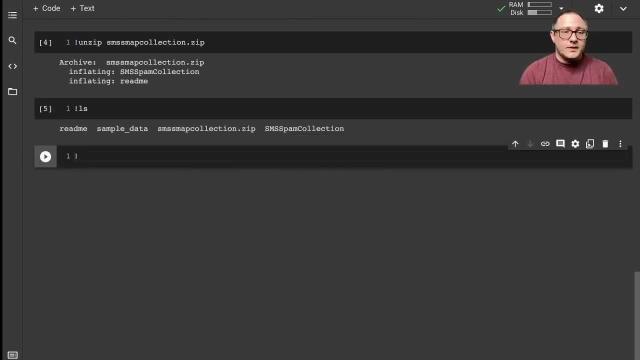 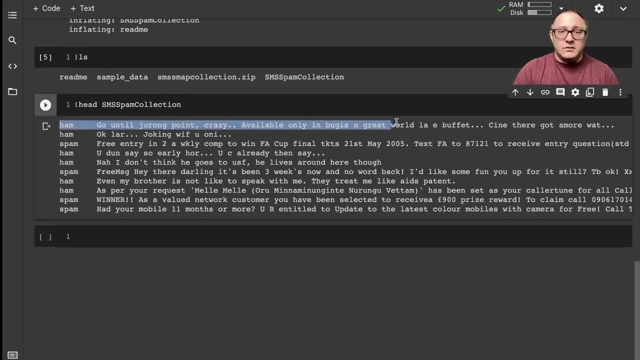 a look and see what format that this data is in. Let's look at head: SMS spam collection- SMS spam. There it is, And so if we look here, we see that this, actually this data, does not have a header at all. Okay, And. 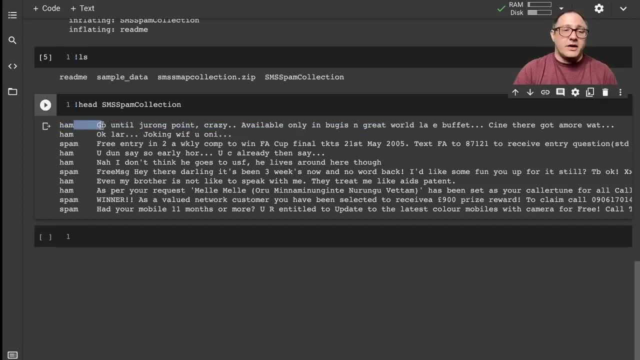 also, my best guess is that this is a tab separated value, So this is going to be a TSV file. So when we go about importing this, let's go through and make sure that we get everything that we need. So let's do import pandas as PD, import numpy as PDF. So let's go ahead and import pandas as PDF. 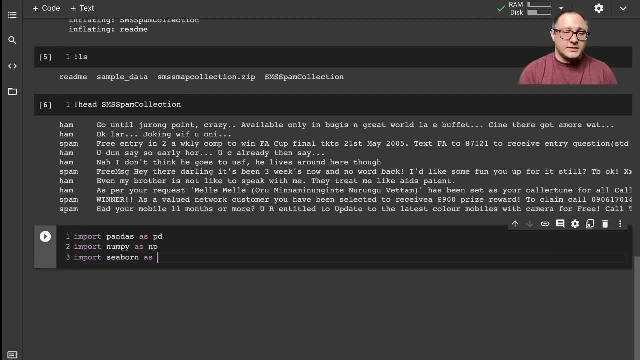 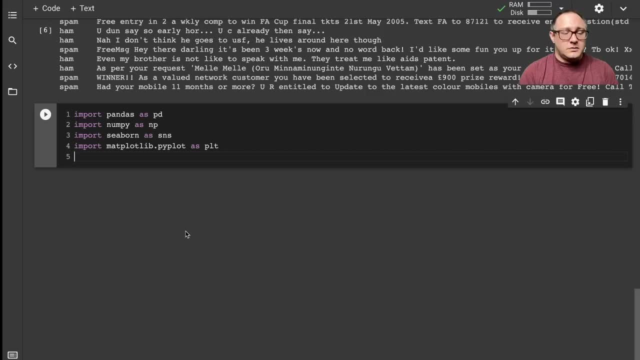 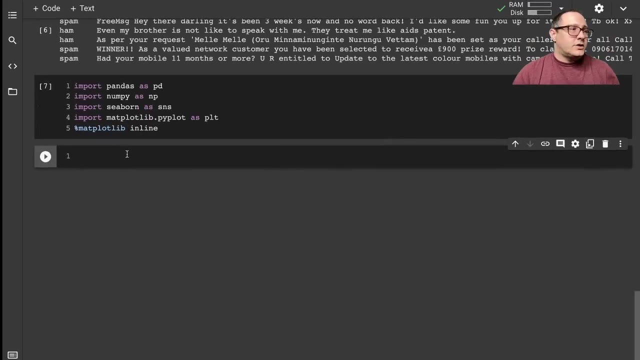 numpy as NP, import seaborn as SNS, import matplot, libpyplot as PLT, And then let's do matplot lib inline And just this. these are just our standards. So let's go on and pull in that data. So let's call this SMS or you know what, maybe we'll just 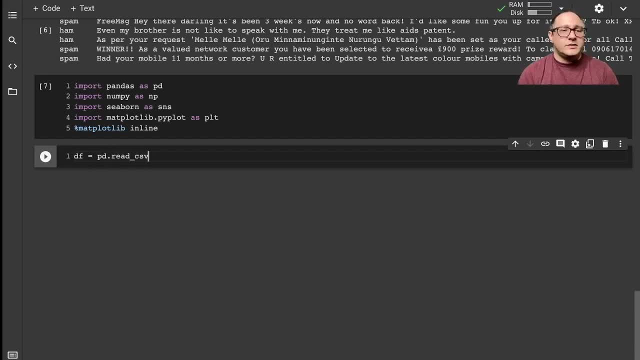 call this a data frame. Maybe we'll just call this a data frame. Maybe we'll just call this a data frame. Let's call this a data frame for now And do pdread csv in here And we want SMS. What was that file? 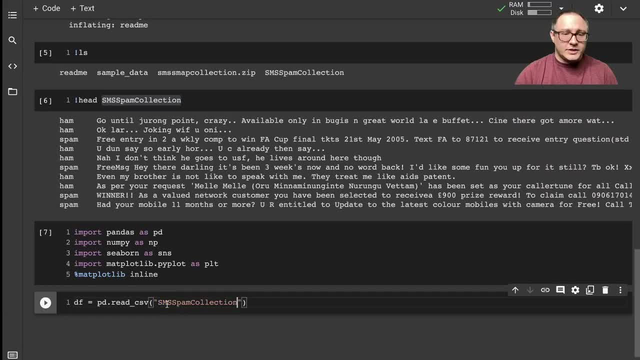 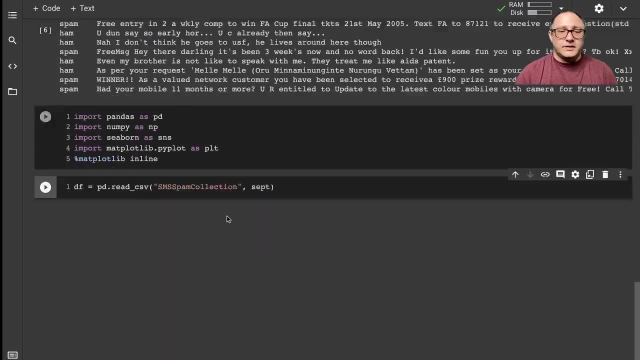 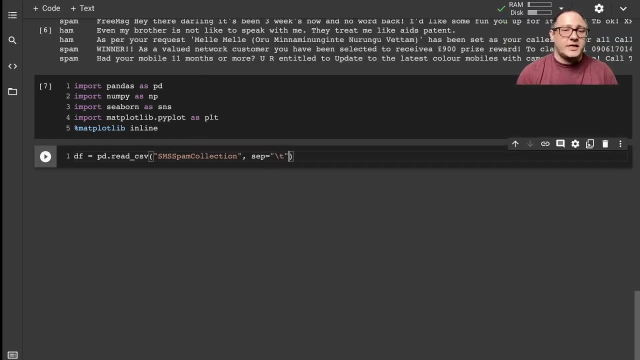 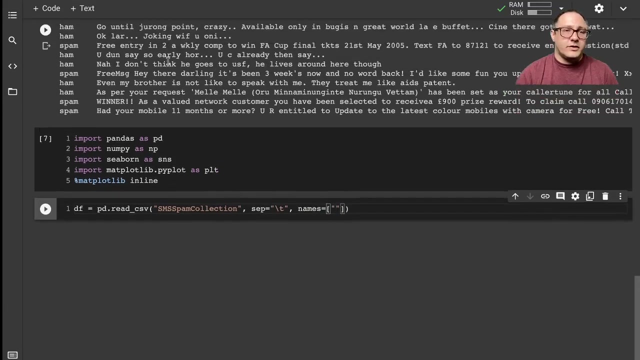 called. We'll just copy this SMS spam collection. Now we need to make sure and do the separator in here. Oops, The separator in here needs to be a tab, So that's a backslash with a T, And then we need to have a label in here, And so we need. so if we look here, we have, for example, this here is: 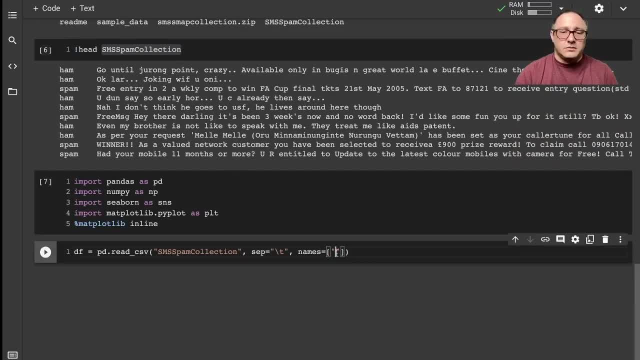 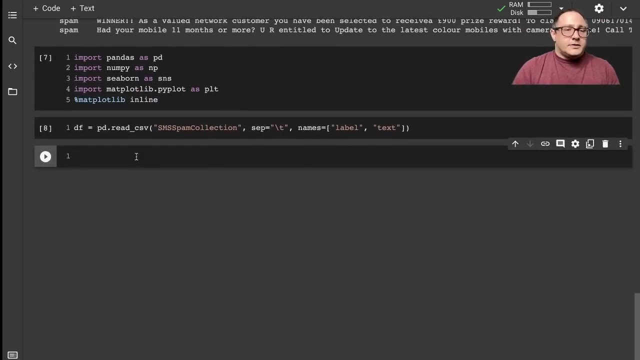 our label, And then we also want in here a message or a text. So you know what? let's do message. No, we'll do text in here, And so let's go on and make sure that that actually looks right, Okay, So. 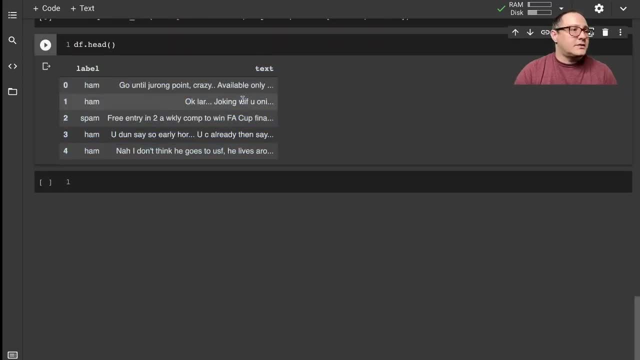 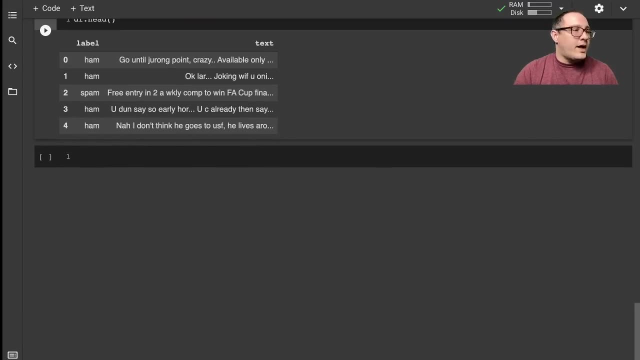 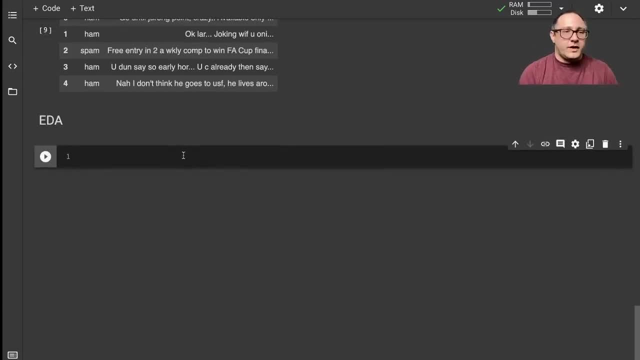 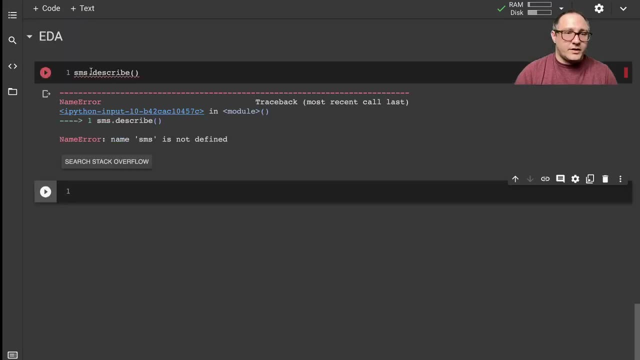 EDA. So we have SMS dot describe: Whoops What did I actually name it DF? I forgot. Okay, So we have full observations. We have two unique, We have 5,169 unique values. So again, that means. 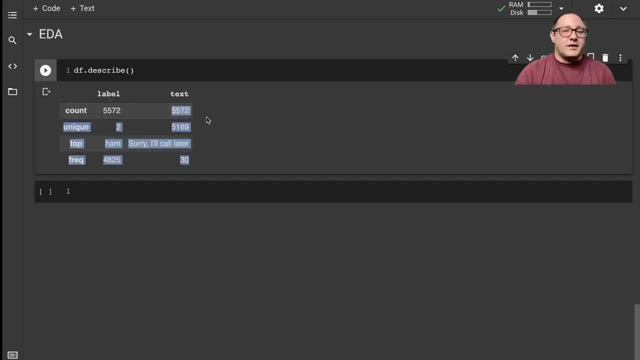 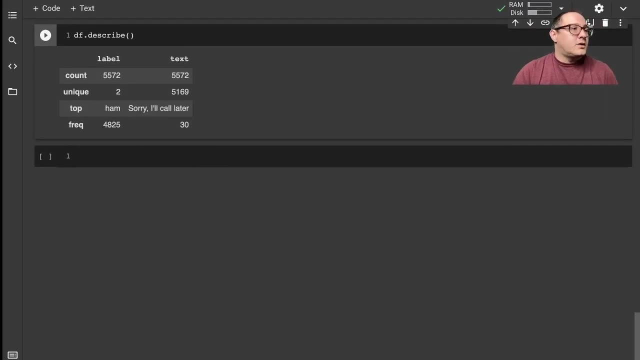 that there probably are some repeats in there. Again, something like K, okay, bye, something like that as well. So let's go on and separate this out, because we do have. if we look up here, we have ham meaning a non. 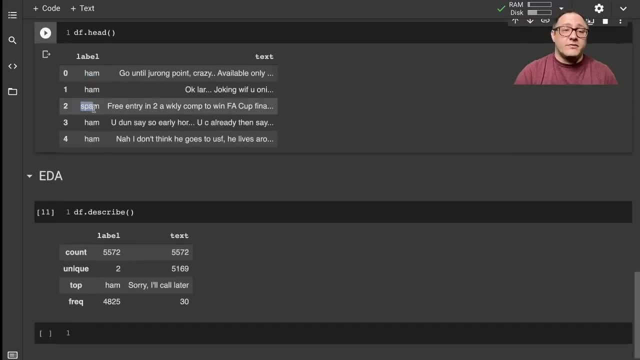 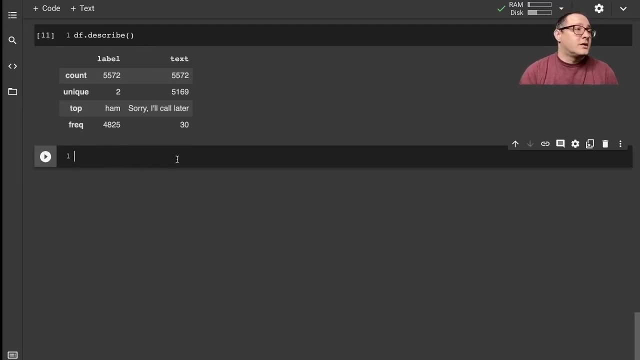 So we have spam item And then we also have spam for a spam text message. This would also work if you're using this for email classification or anything else. So let's go on and do messages, Oh, not messages. We want DF dot group by in here and we're going to group by the label. 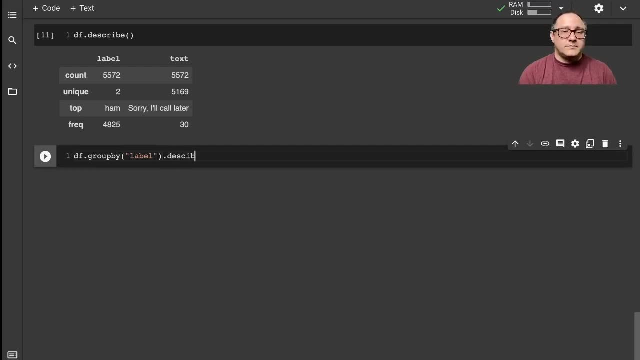 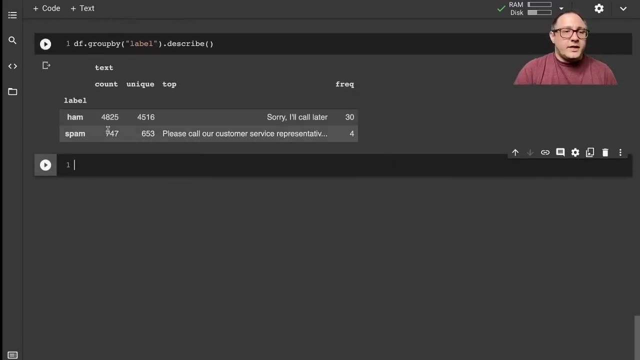 And then we want to do our describe as well And take a look. So again here, notice that this is actually a pretty unbalanced data set We have a majority are ham and less so are spam, And again, I'm kind of hoping that that's the case. 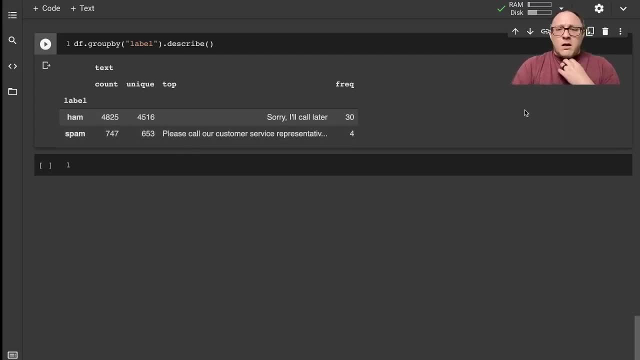 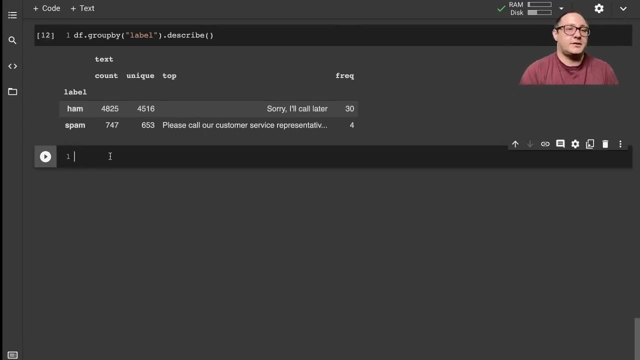 Again, depending on your email. Oh bless me, Sorry. All right, So let's also maybe look at doing some more spam. So let's go ahead and do some more spam. So let's go ahead and do some more spam. 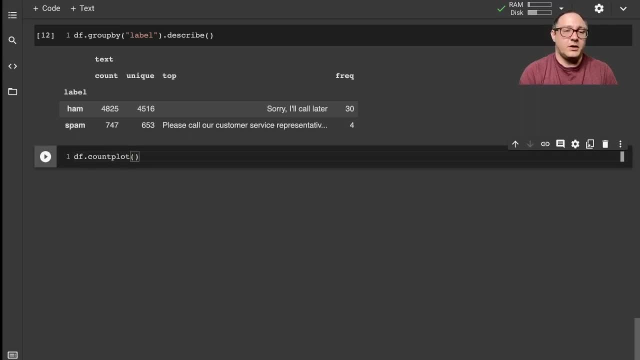 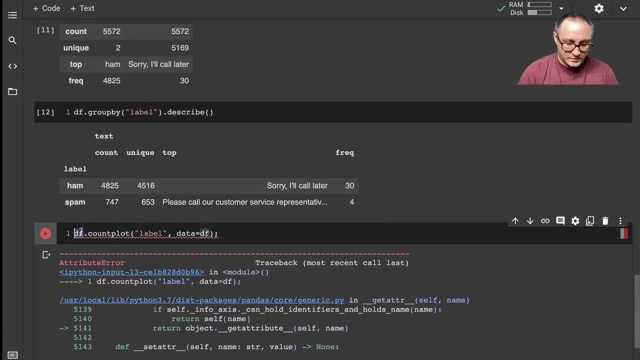 So let's go ahead and do some more spam. So let's do some more spam. So let's do something like df dot count Plot in here and we want here label and we'll have our data's to DF. Whoops, It's because I'm SNS. There we go. 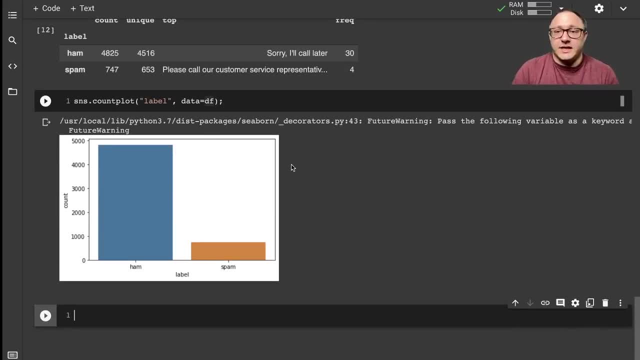 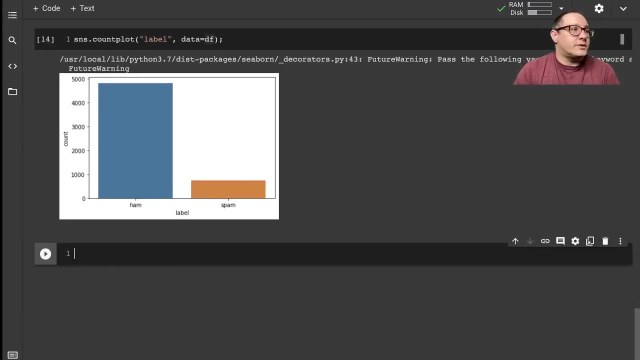 And so, again, we can also have a nice visualization there, seeing that, again, it is a majority of ham. And we can also have a nice visualization there, seeing that, again, it is a majority of ham. Um, so another thing that we're going to need to do is start to do some, uh, feature engineering. 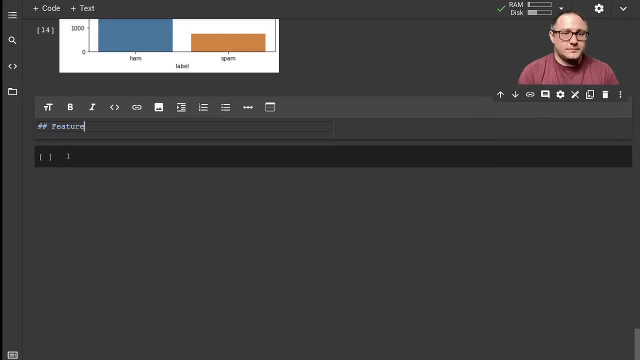 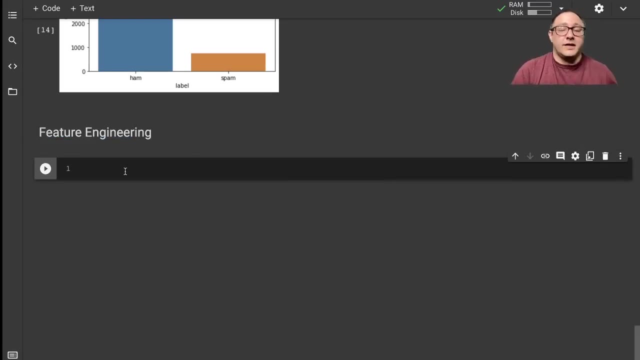 in here. Um so, um again, some things that we want to do in here is to have the length of the message. Okay, So how long is the text message? Uh, that type of thing, or maybe later on if you guys are doing tweets or something. 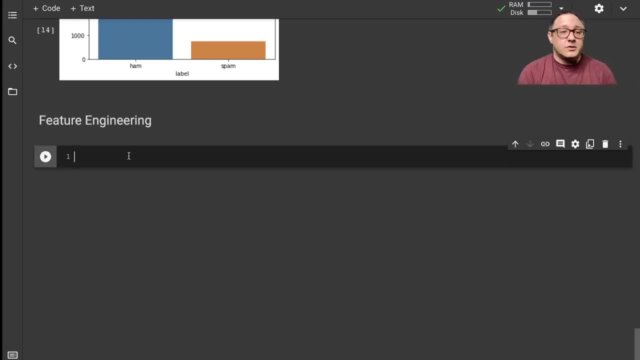 how long is the tweet, how long is the email, et cetera. So let's go on and do um, call this length in here, And we want uh DF text and we want um to apply and here the link function. 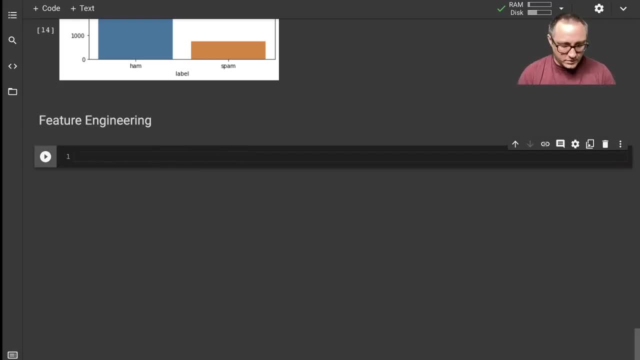 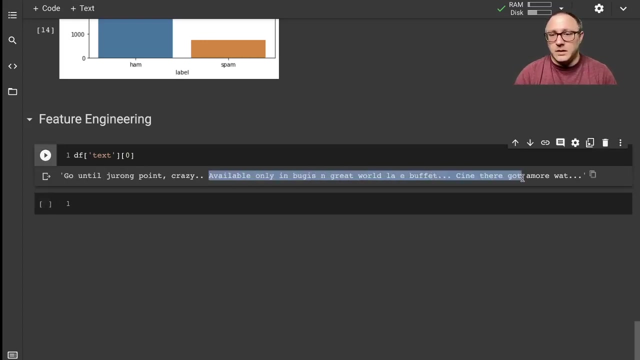 Okay, And maybe, maybe I can show you guys an example before, oops, before we do this. So if I do um DF, uh text, um zero, Okay, So you can see here: uh, go until the wrong point. crazy, uh available only in. uh blah. 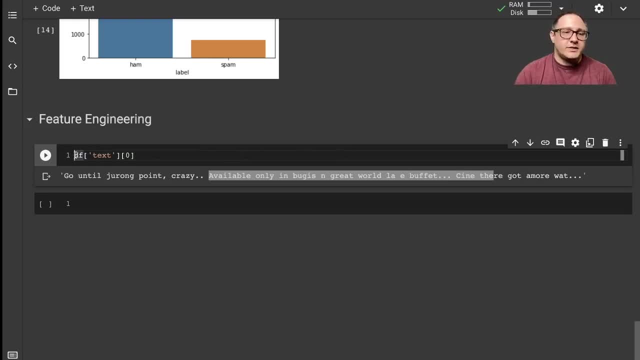 blah, blah, blah blah. Okay, So if we want to take and we want to see how long the string is, we can do length on side this and it will tell us that it's a hundred and 11 characters. 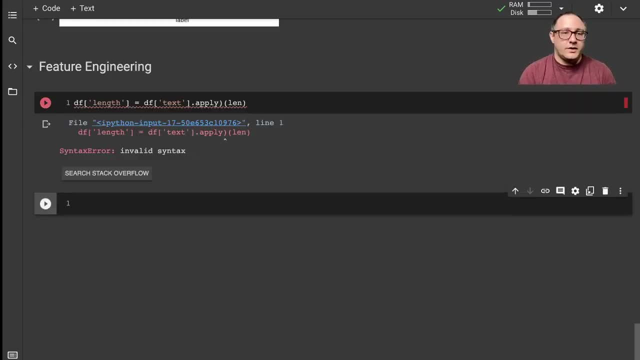 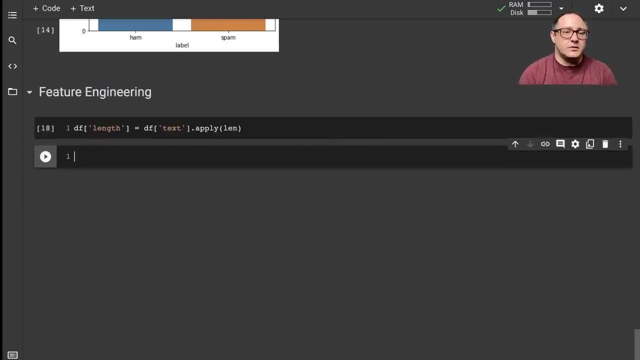 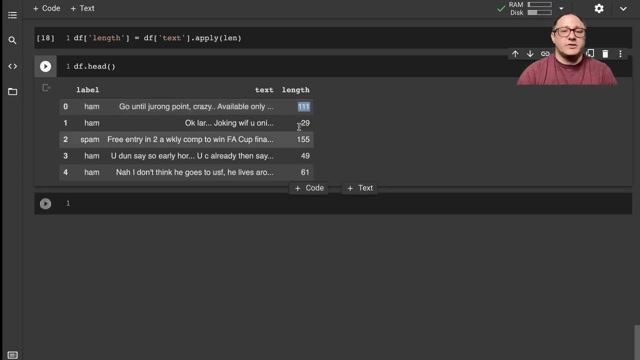 Um, so let's go on and run this Whoops. Okay, So we can actually go on and take a look. So, uh, now we can see here again that one wound up being 111 characters and we went through and grabbed the length of each of them. 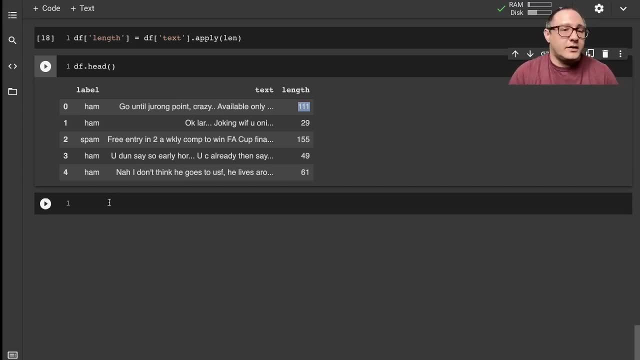 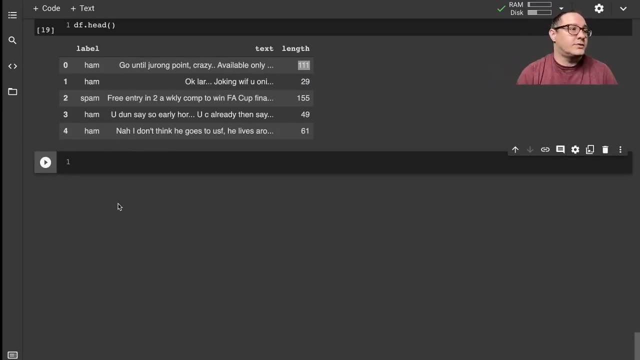 Um, let's go on and also take a look at the histogram for that particular um, for that particular item. So let's do um, what S and S dot uh display, Okay, Okay, So we'll do this plot, uh, and we'll do this on the length and we'll do uh. data is equal. 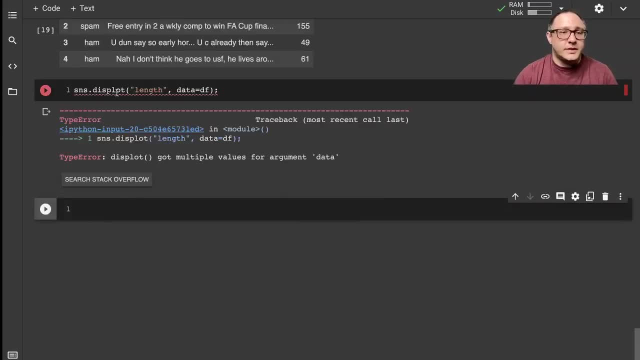 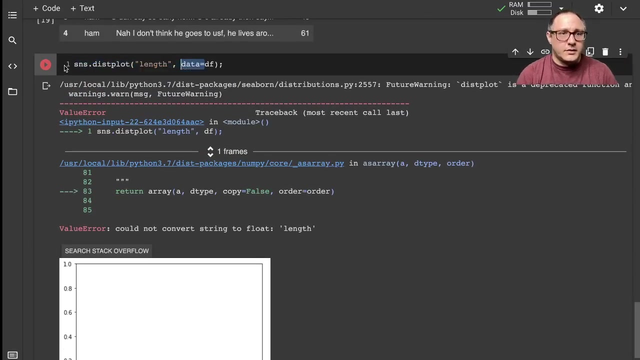 to our DF. Oops, And it's dist plot. Oh, and what happened in here? Let me actually just delete this and hold on. What happened in here? All right, Let me cut this all out. S and S dot Dist plot. 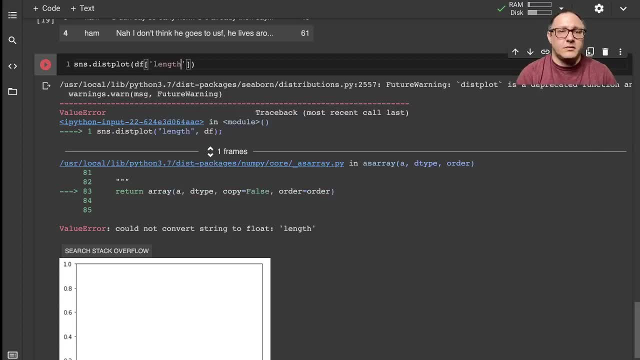 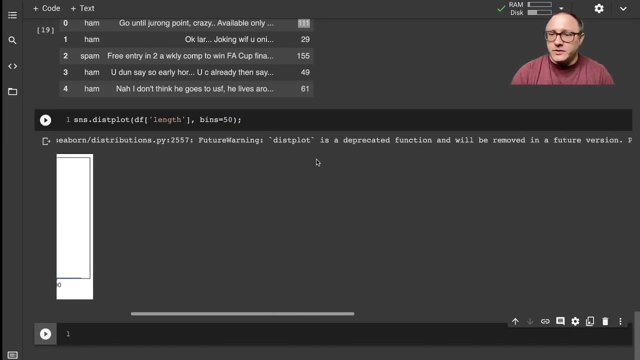 And this takes in. okay, we can just do DF length in this case, Um, and let's have our bins, uh, equal to 50. Okay, And we see here that, uh, well, this is going to be depreciated. 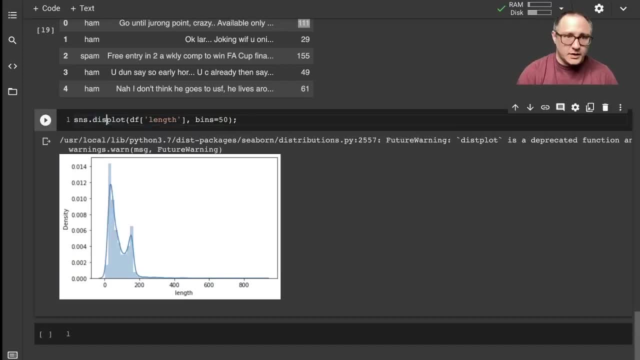 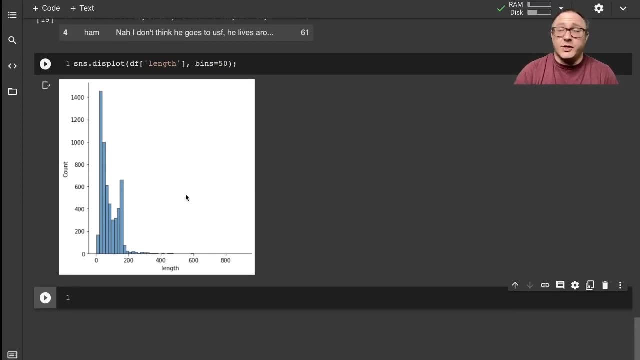 So what does it actually want me to do? is this plot? Okay, So I will go back to this plot, Okay, Okay, So I'm going to go ahead and delete that. This is definitely um skewed. Okay, A majority of these text messages are pretty long. 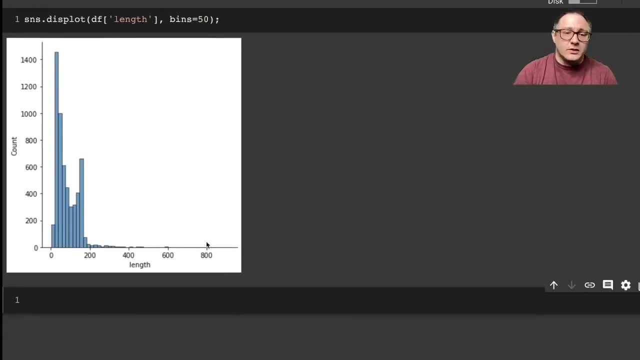 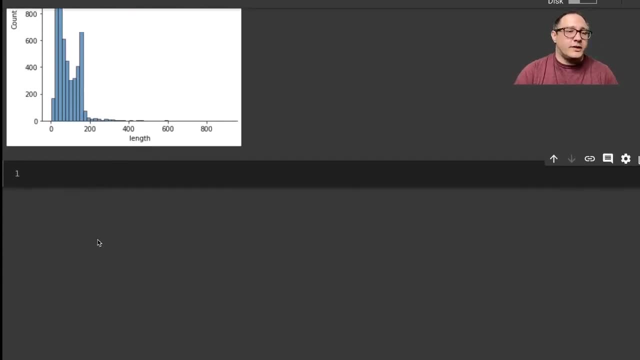 Okay, And then they kind of Peter out again. Apparently, we have some really long uh text messages in here, which I find is kind of strange. So let's maybe actually go through and look at um at the length variable a little bit. 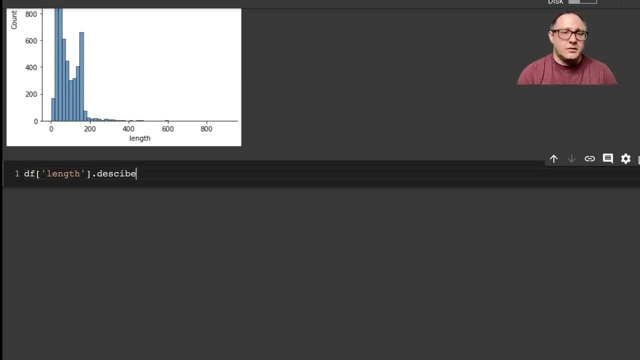 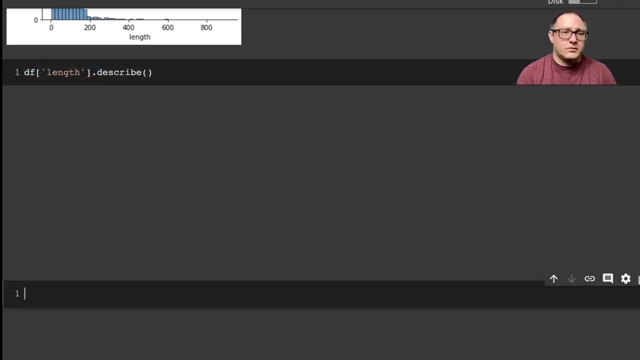 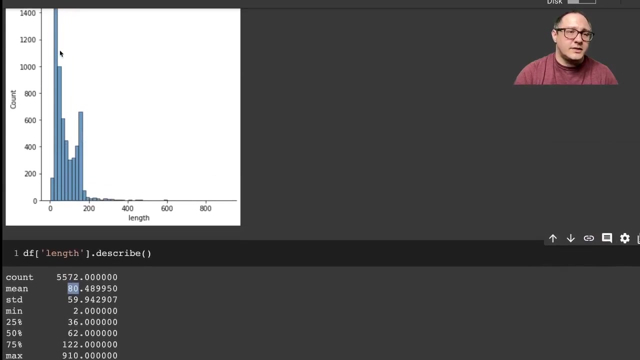 and uh see what exactly is going on. Okay, What's going on? And again, my, my fingers are not wanting to work today, are they Okay? So This is our count, or mean, is around 80.. So that's, that's what this bad boy is, is probably around here somewhere around 80.. 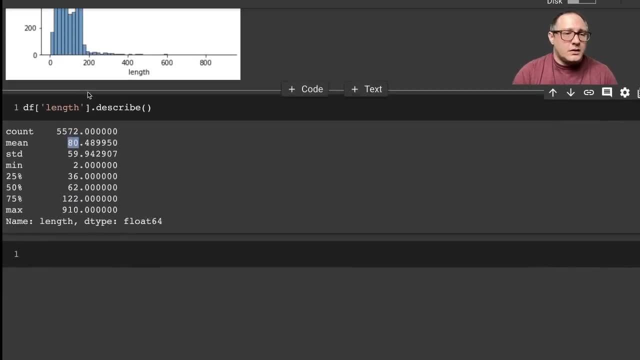 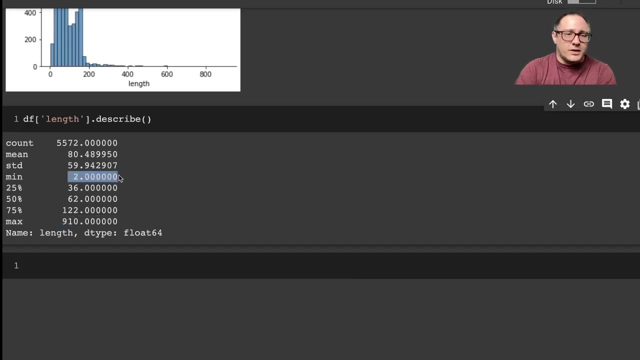 Mm 80.. Yeah, Somewhere around here. Uh, our maximum is 910 characters. So those are some of those are pretty long, long. let's actually see what's going on with this maximum value in here. minimum is a two, so probably something like okay. so, but let's, let's, let's take a look at. 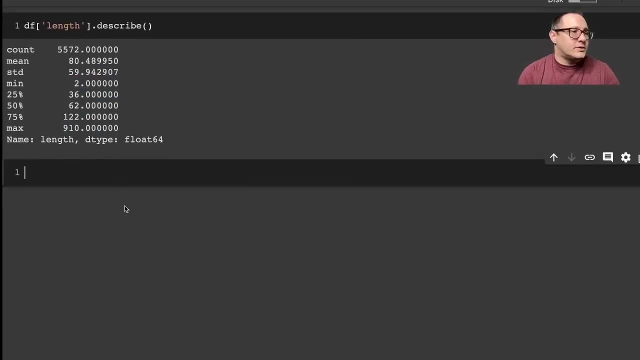 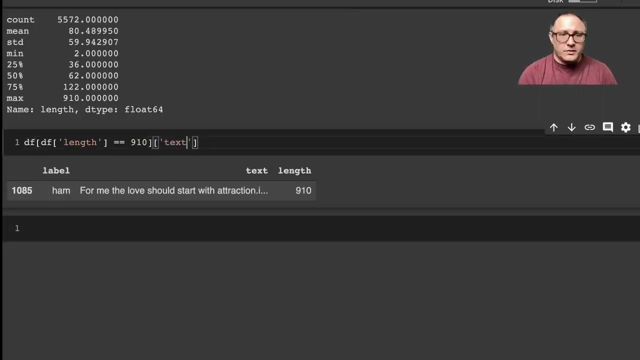 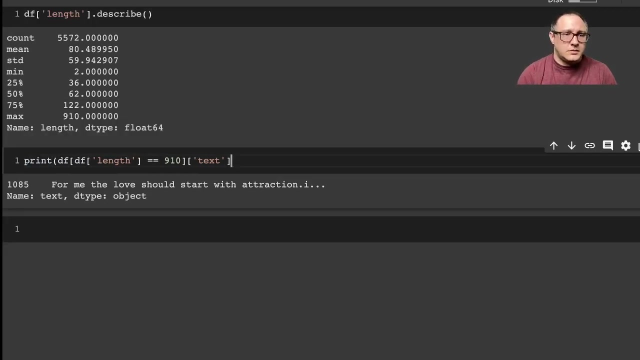 that first message. so let's do data frame and we want what length is equal to 910? and let's go on and grab in here the text and let's print this. no, I want it in a different way. let's go through and do what's a better way to do this. 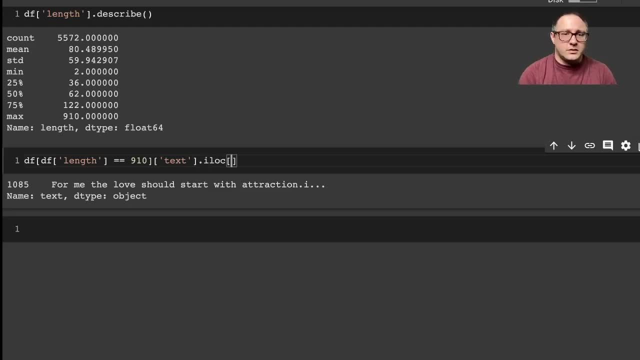 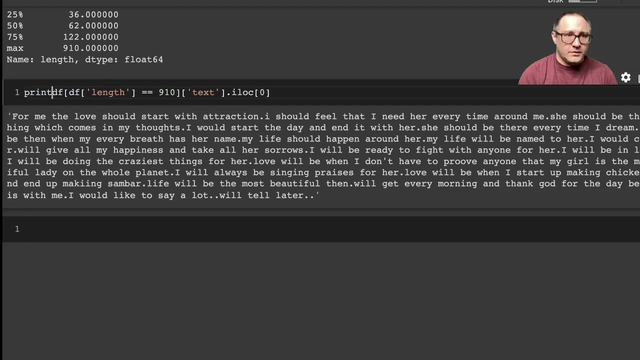 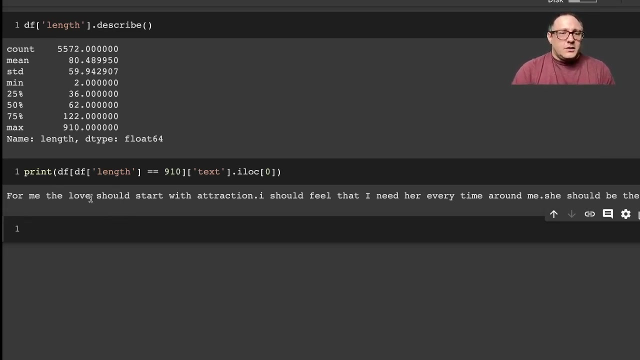 let's do text dot. I loke of zero, all right, so this is. this is the whole text in here, and maybe let me print it out so that we can see it. no, I don't like it like that, but we can kind of see it here, so so again here: basically looks like they're writing: um, maybe a love. 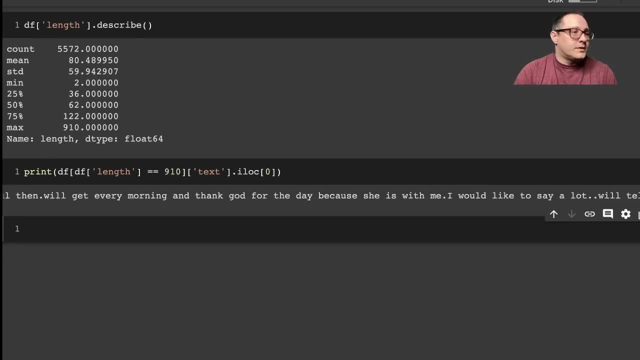 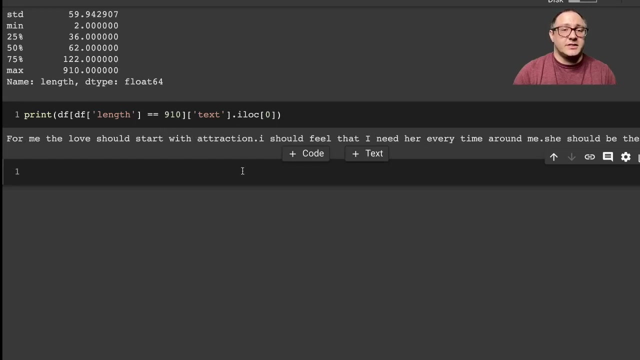 poem or something like that, nice and long. so that's fine. um, but again, let's, let's maybe see something, maybe if there's a distinguishing features between spam and ham, because again, I don't think that this particular one is a spam feature, but it is kind of interesting to see these nice texts, you know what? maybe? 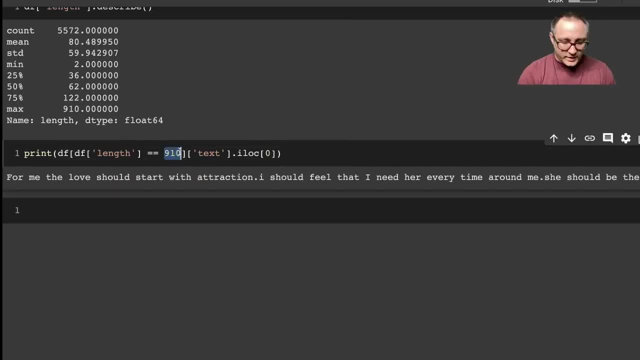 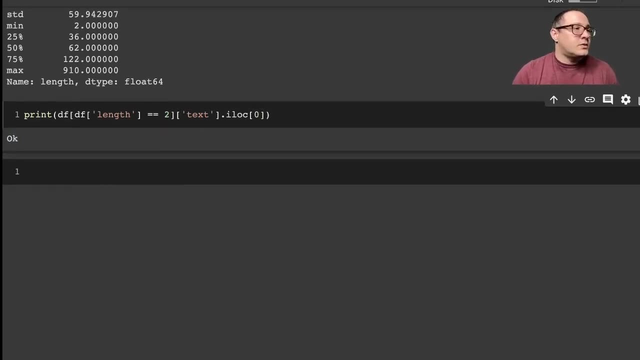 let's look at. let's look at one more, okay, and let's look at those that were at two. so see, and again it is okay. so let's go on and maybe take a look then at what do we want to see here? all right, let's let's separate them out by label so I can go on and I can grab. 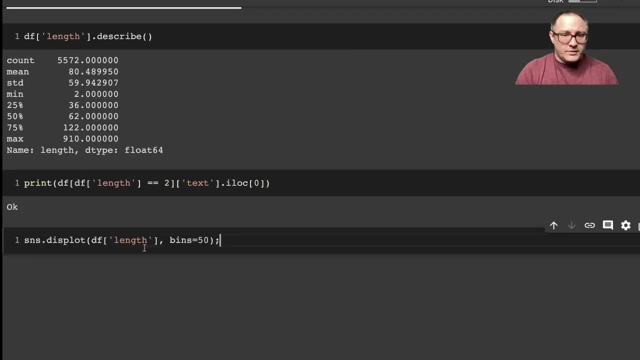 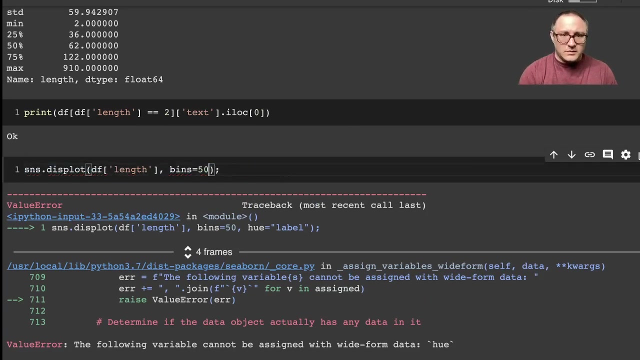 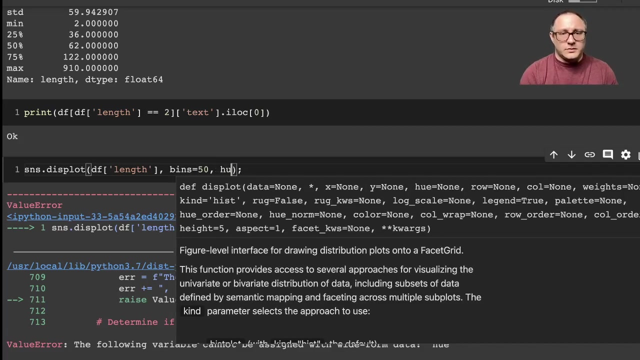 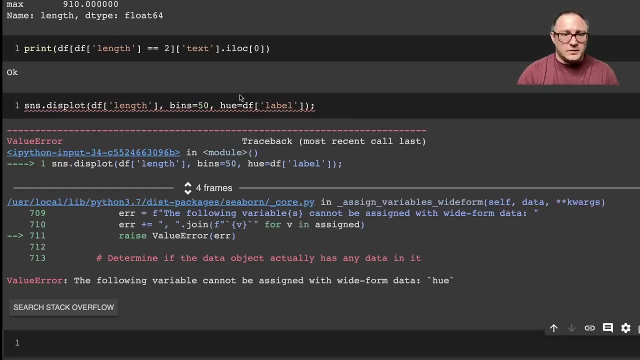 this, put this down here, and then we can do something like: um hue by label. no, does this one not have hue? I forgot about that, mmm. no, it does have hue. hmm, no, it does have hue. hmm, no, it does have hue. oh okay, so hue here and let's do DF label. it's still not gonna like it. 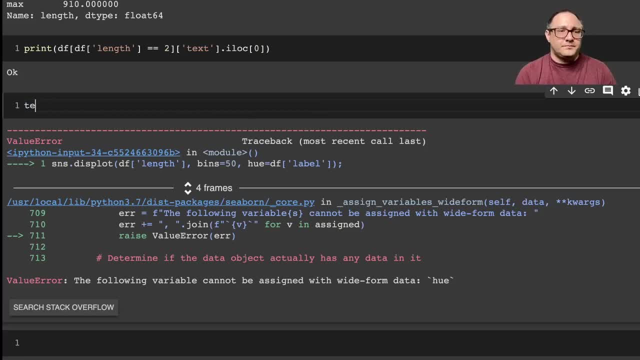 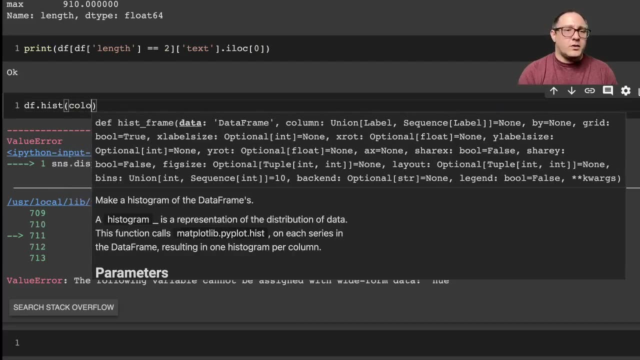 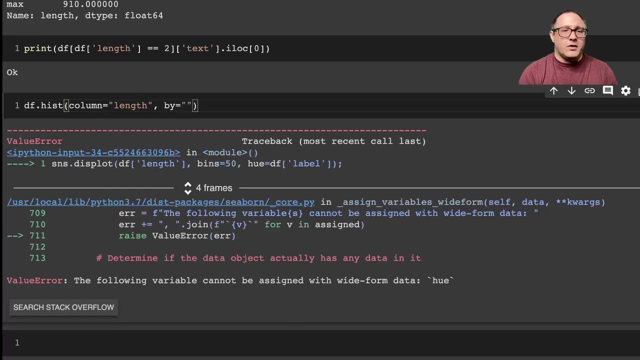 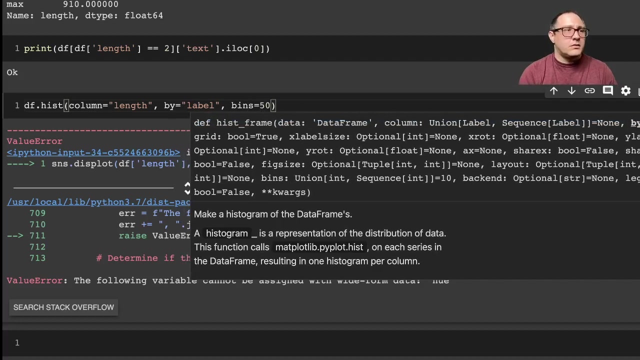 oh, because it's white. so then let's just do it with um, let's do it with just the plot mechanism. I'm here, histogram on our column here to be length, we want this to be by, by our. we want our bins here to be we had 50 before, and then let's change our figure. 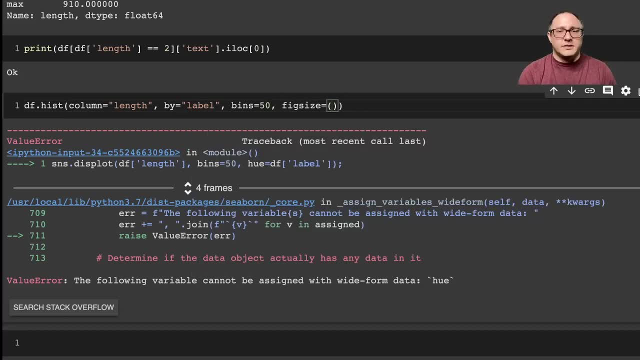 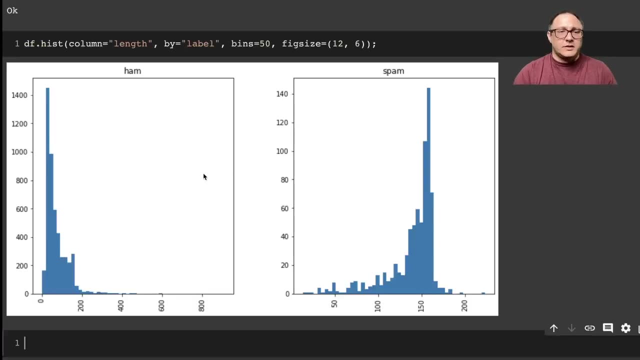 size, size here to be something like 12 by 6. let's see what we have here. all right, so then we definitely see that there's a definite distribution here that we can see. ham has a tendency to be very, very short in nature. so non, non. 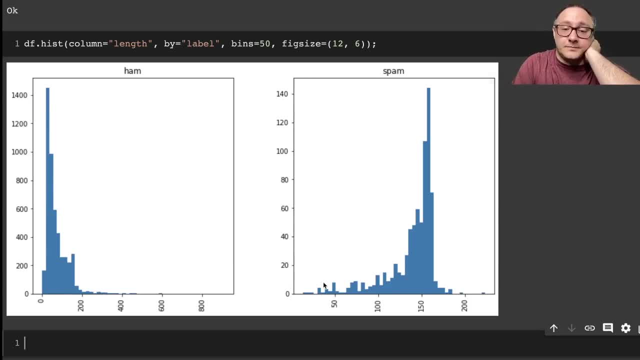 spam is very short in nature. now, spam features tend to be, on the long end, quite long, so around a hundred and a hundred and fifty. okay, for for their average maybe a little bit more than that, hundred and seventy. so again, this tells us that length is definitely going to be useful. 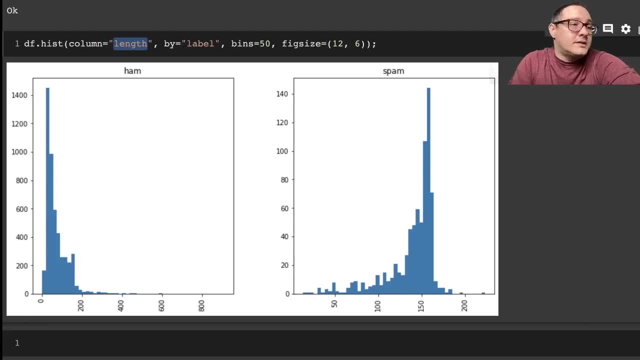 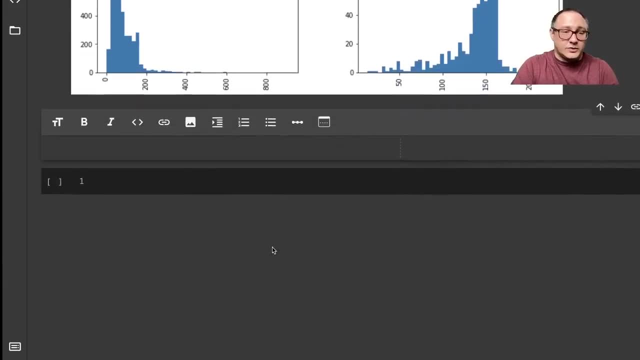 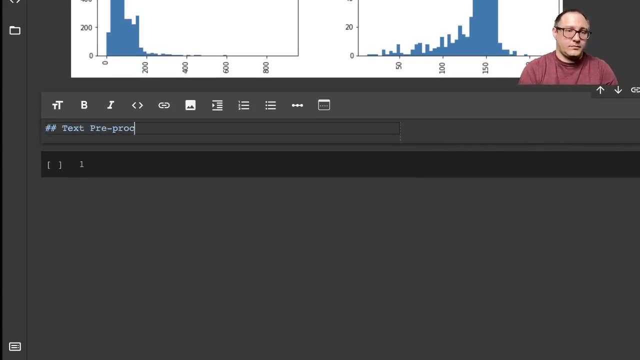 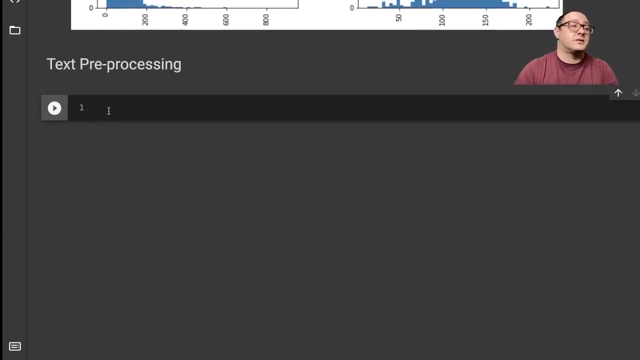 you when we're doing some sort of prediction analysis. so we're gonna have to keep that in mind. so let's go on and start our actual textual analysis and our text pre-processing. so text pre-processing, we're gonna need to grab on a couple things. so the first thing we want to grab is some from NLTK here, the corpus. 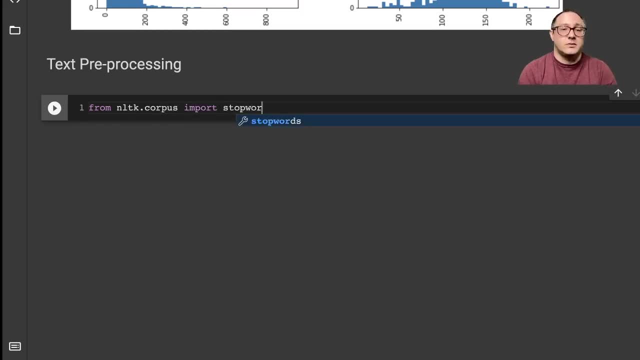 we want to import stopwords. so stop words are actually again something that's like very, very commonly used. so I me, my we are is. so let's actually maybe, instead of me talking about them, let's actually take a look at them. so we want the words, we want to make sure that we're looking at English and this. there are multiple. 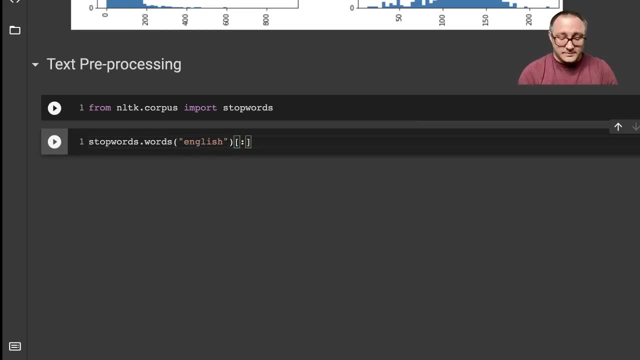 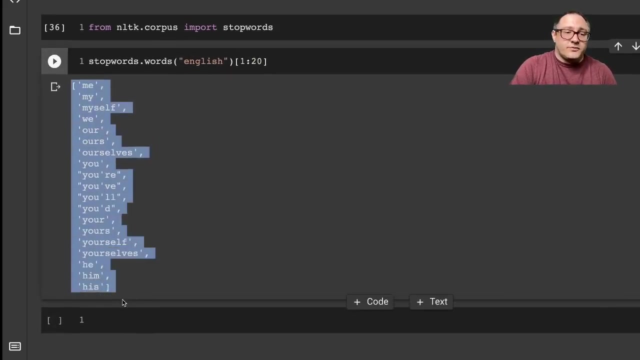 language. so. so then don't. if you, if you want to do natural language processing and maybe another language or something, feel free to okay, there are several. I've even done textual analysis and Chinese before. so again, those are all available to you. so here we can see here that this is the first 20 of the stop words, and so we. 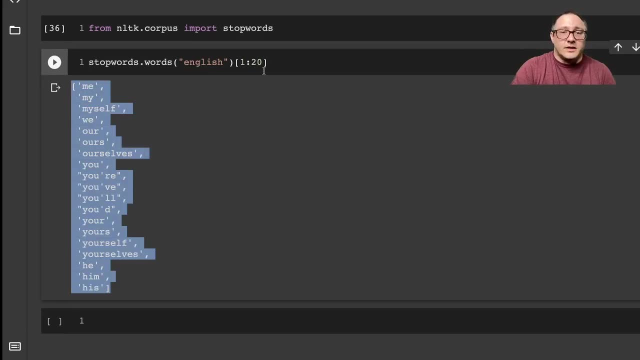 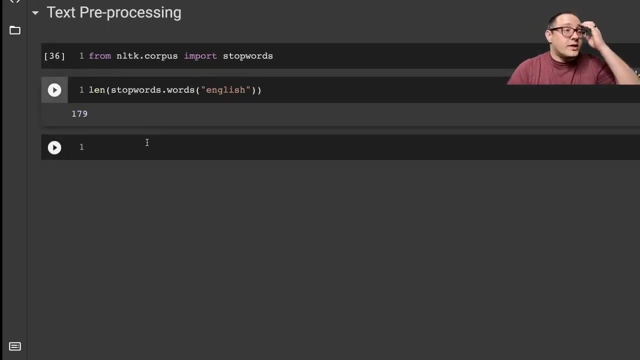 have again it's. these are all, for example, pronouns or something like that, but let's also look and see, for example, how many stop words there are. so here we have: it has just 179. you can also- probably won't do anything about that today, but we can do something like add in our own stop words or something like. 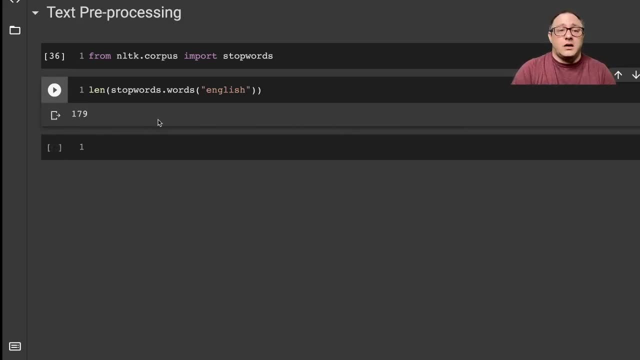 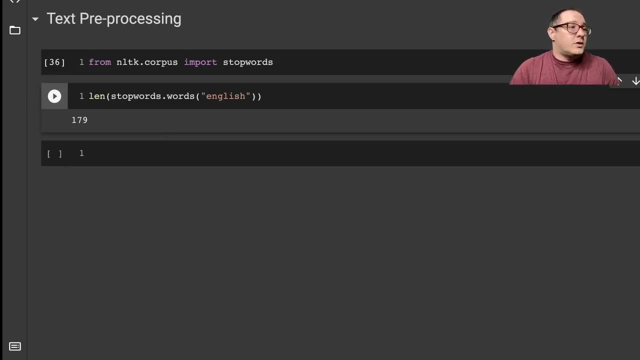 that again. once you start doing your own higher-level pre-processing, maybe you have a specialized data set that you use for your company or something. so another thing that we actually need to go on and do is actually make a bit of a function here to pre-process the data. so our goal would be, for example, is to remove 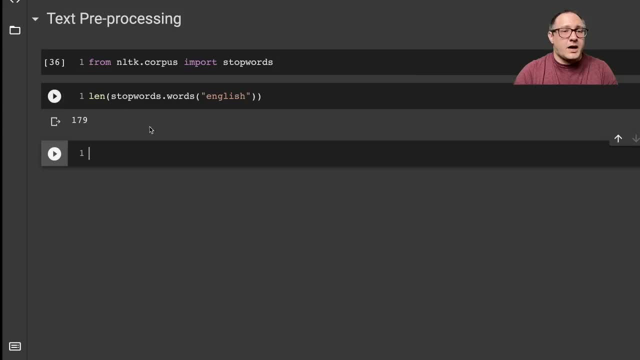 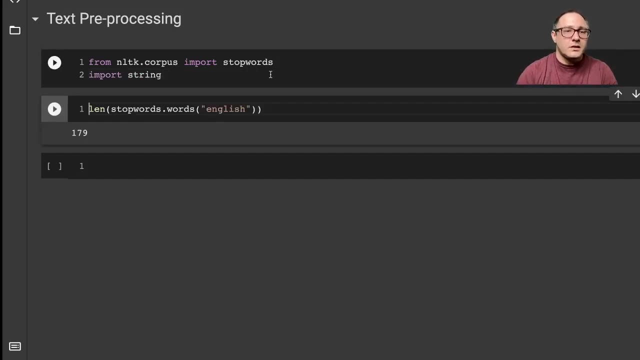 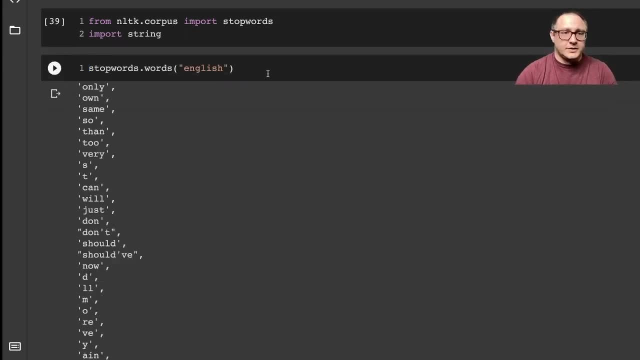 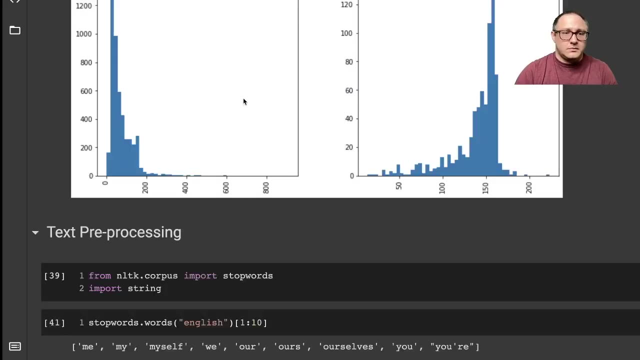 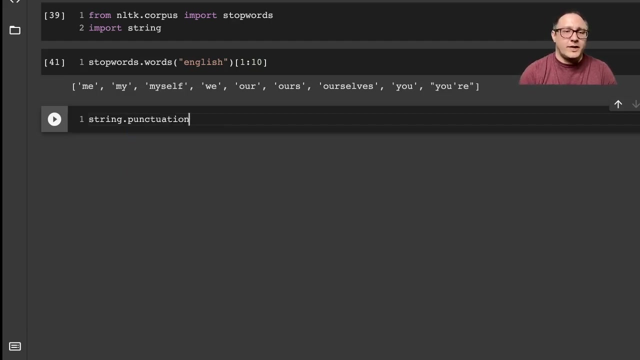 me actually have that example, full example, up so you guys can still look at that. none, zero through. let's do 10 for now, okay. so then you can see the whole thing now. another thing that we have is from the string package we have a punctuation, okay, and so here you can see, here this is a. all the punctuation is. 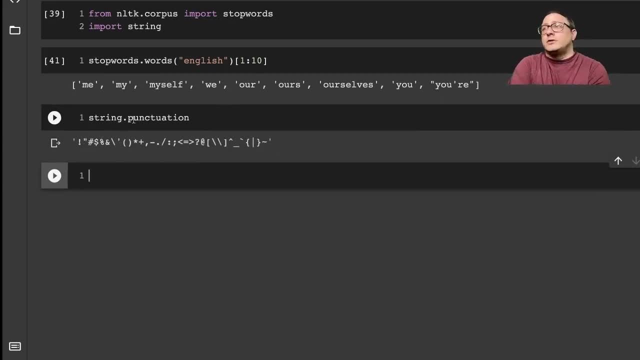 the punctuation that we would wind up having. we need to also remove punctuation. Okay, So we want all of the periods, the dollar signs, the percent signs, all of that stuff needs to be removed, Okay, So let's go on and make a function that actually removes the punctuation, and it maybe 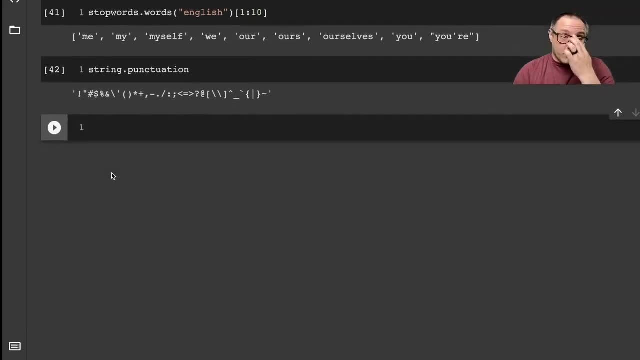 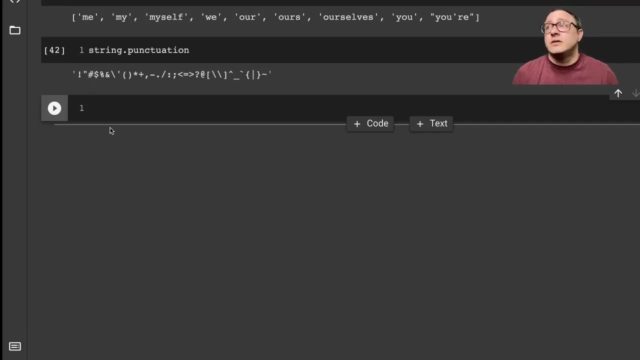 does some text pre-processing Now, as I've talked about before, okay. when you're going to be reusing something a lot, particularly with text processing and those types of things always make a function. Remember to keep things dry Okay. Dry Okay. That means here is don't. 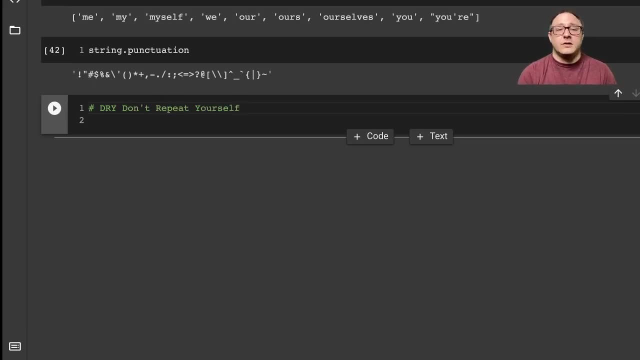 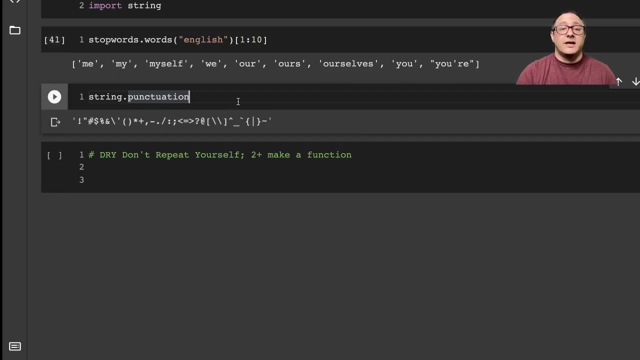 repeat yourself: Okay. So the cardinal rule is: if you do it two times or more, make a function Okay. And so again this type of function, particularly when we're doing this text, pre-processing, getting out stop words, getting out punctuation- you're going to do it every time, So you might as. 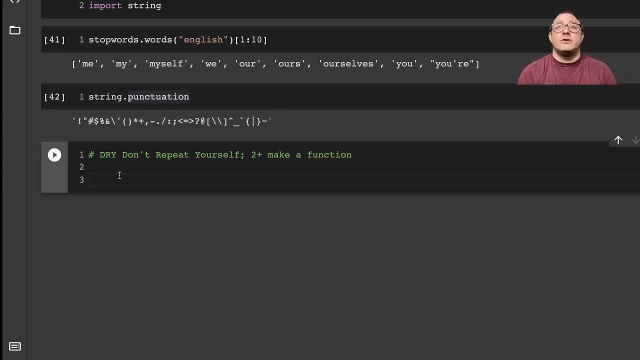 well, create a function for it, And then that way, all you have to do to add special stop words or add special punctuation, or something that you want to remove is very, very easy to do by updating the function. So let's call this text processing, And this will take in. 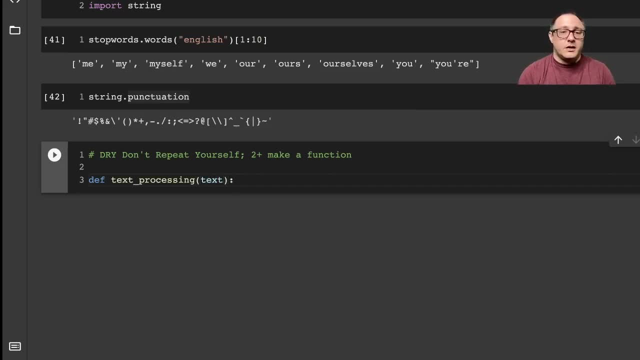 some text in here, And you know I'm not going to use text. I'm going to say, yeah, text will be fine. And so let's see here What do we want it to do. We want to remove punctuation. Now, I'm not going to do this in. 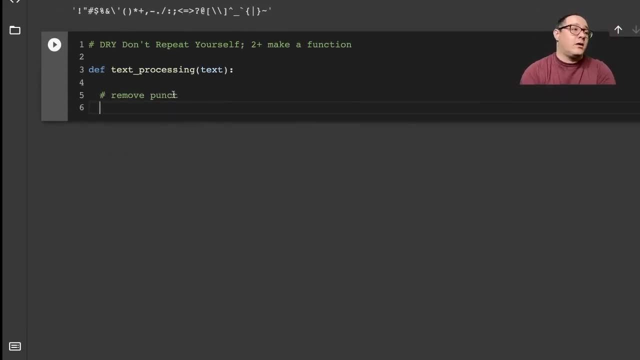 I'm not going to make up a full documentation on this. I would go back and do that later on. Um, so, um. so here let's do um, uh, a character for character in um the text, if the character is not in. 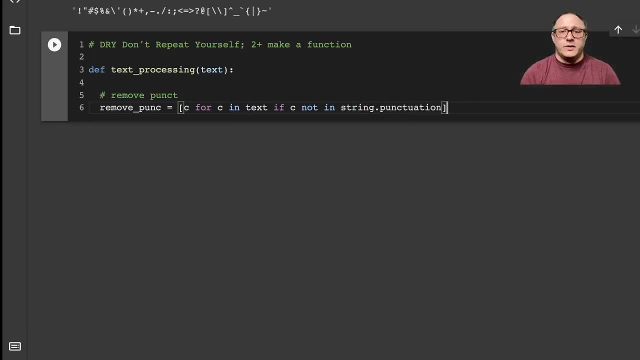 string punctuation. So here this is using um- a list comprehension- in order to do this. You can also do it in a um in loops, if you, if you, so choose, but I would, I personally prefer to use um, this uh punctuation. 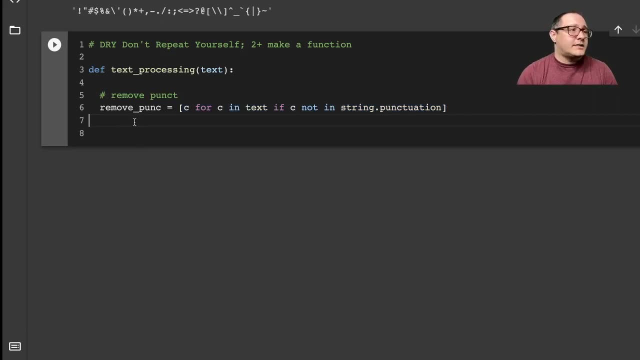 or this uh list, comprehension? Uh. next thing we need to do, though, um, is actually to join them together, Cause this actually puts them into um a list. uh, join, um, join them together in here, And so we will overwrite this. remove punctuation, and we'll do. 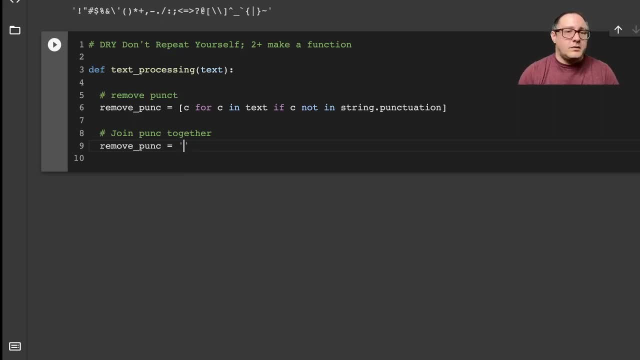 something like: uh, we want it separated by nothing here, and we'll do dot, join, remove punctuation Uh. and then the next thing that we would want to do here is: um, remove stop words, Uh. and so here we would want to make a return statement and we'll say word for word in: uh, our. 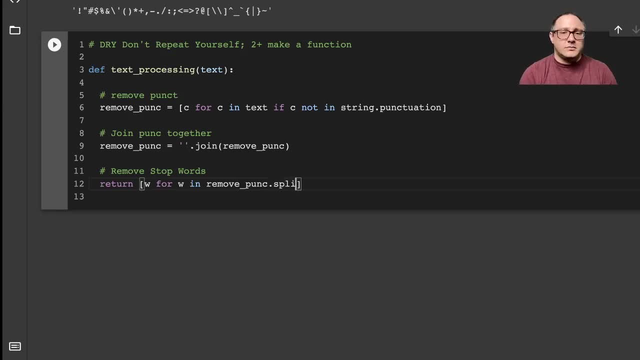 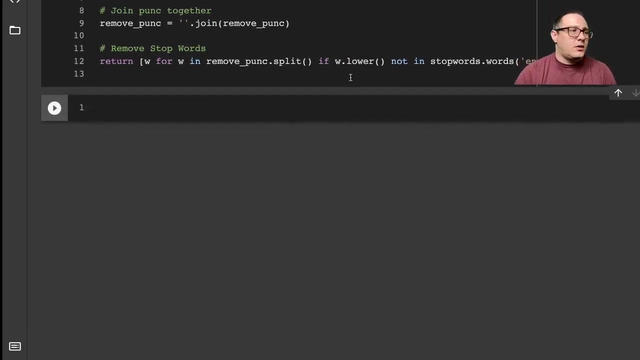 remove punctuation dot split If uh word uh word if word dot lower uh not in co eles da que stop words or two words um here and we want English, So let's go, Let's go on and actually let's take a look at our original data frame really quickly. 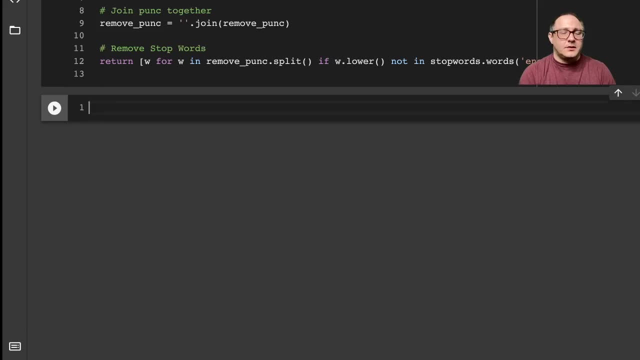 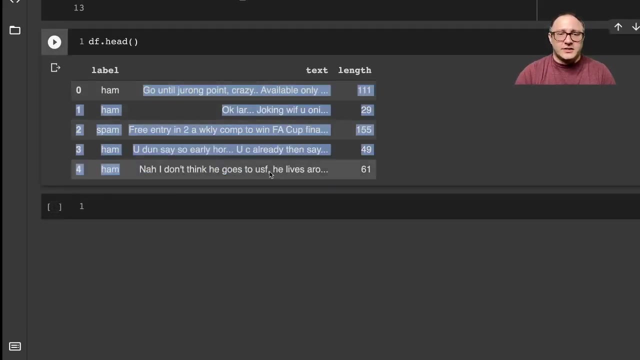 And let's do something like dfhead here, And you can see here that our text has all of this Okay, so they're all looks pretty long. Now there are some issues with this. You can see here that there's a lot of text speak that type of stuff. 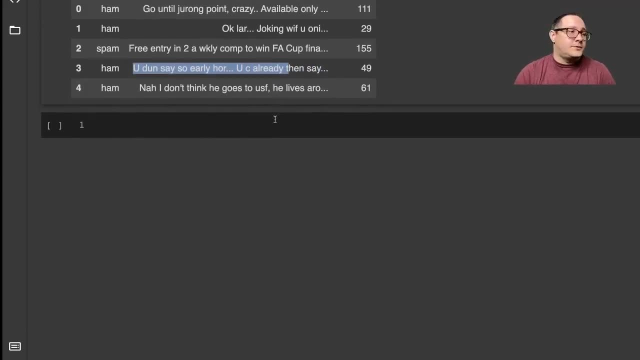 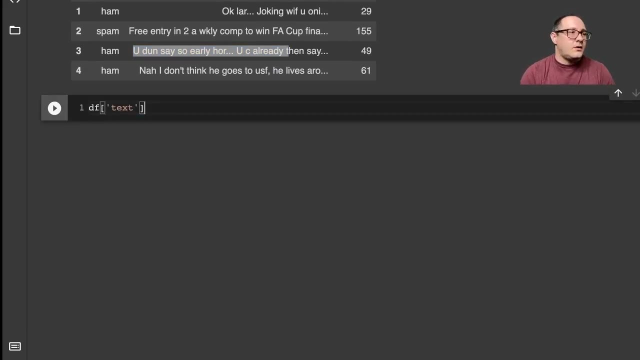 So you may have to have specialized processors for that. just to kind of give you an idea. Now let's take a look here at our text messages. here, dot apply our text processing. I probably should have done that on a subset, but it's okay. 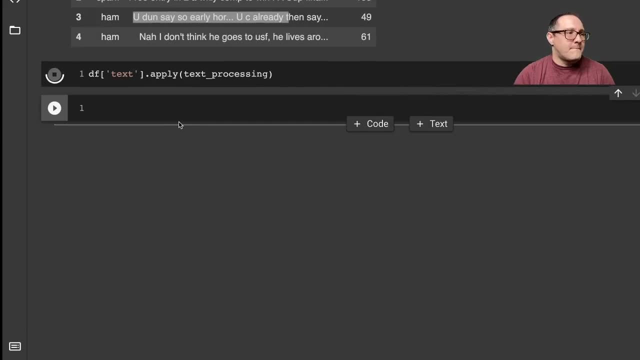 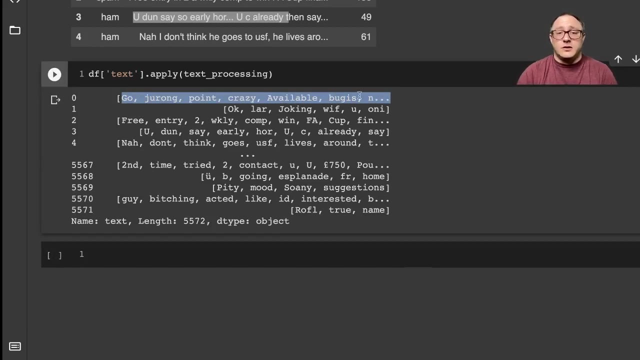 It'll take it just a minute here to run. So you can see here that it split everything into these tokenizations. So tokenization in this instance it's split. It's split it up by its name. Okay, now there are several prebuilt models and stuff that you can do this as well from the NLTK package. 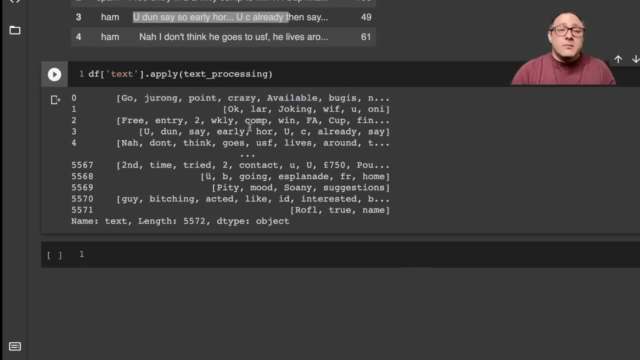 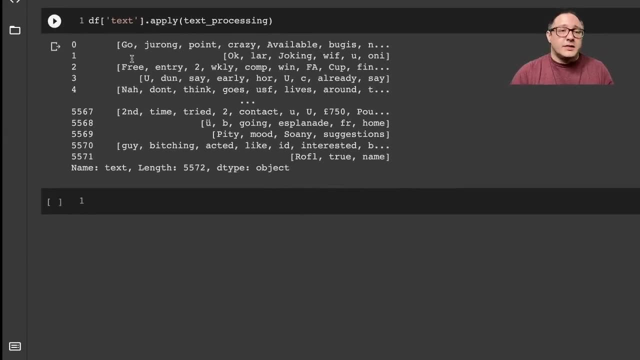 There's even some other packages as well that you can use, But sometimes it's best just to be able to write your own to be able to control the process. So here we can see that it tokenized everything for us, So we also need to do some normalization in here as well. 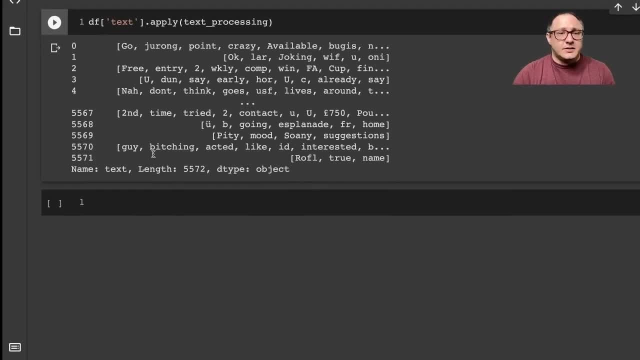 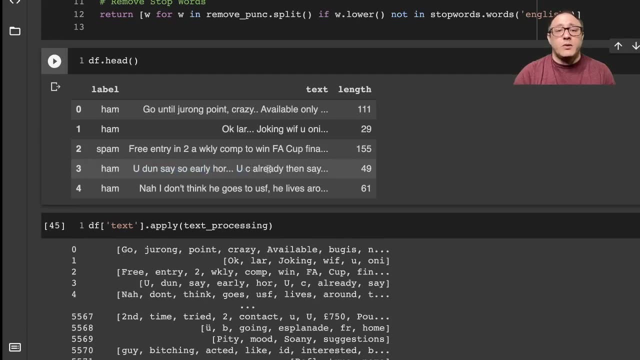 So normalization again is, for example, this: you done say something like that And you, for example, needs to be Y-O-U, those types of things. There are several ways to normalize And you can do something, such as stemming the data using parts of speech. 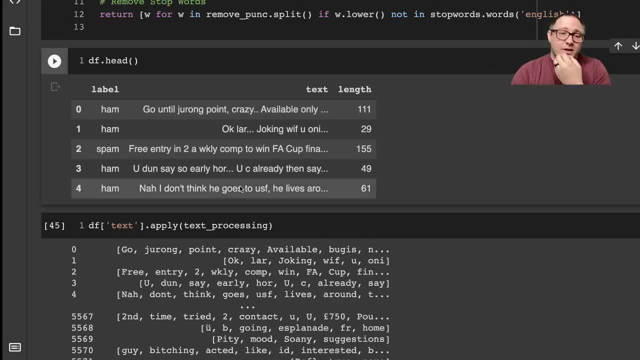 We're not going to cover that in depth today. Okay, this is just kind of a basic introduction to things. We'll maybe do that in another video. We also then need to do, for example, some vectorization. So vectorization in this way can do counts. 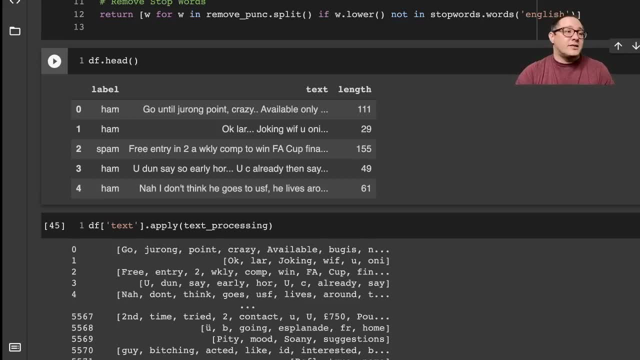 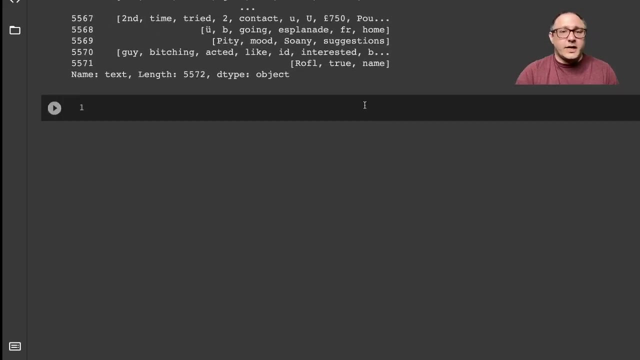 We can weight the counts, We can also normalize the vector units, And this is again making so using a count vectorizer. So let's actually go on and do this, Okay. so let's go on and do the vectorization process here. 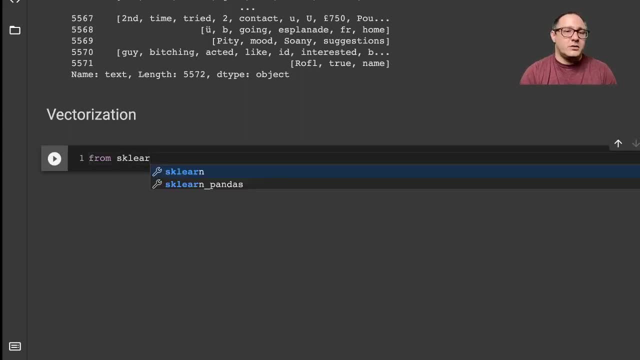 So from sklearnfeatureextractiontext, import the count vectorizer And we'll create a transformer. And this is actually from a bag of words. Okay, so a bag of words. just think about, you have everything, all your words, in a bag, and you kind of just go and pull out and take this. 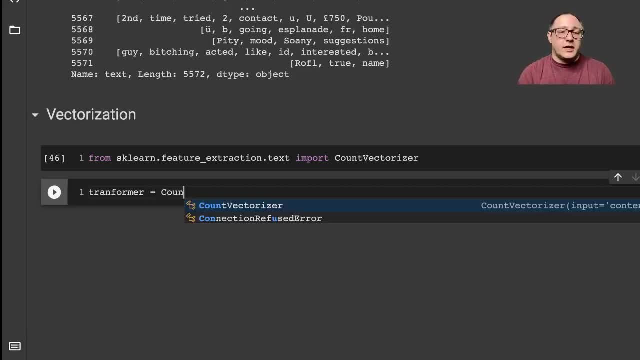 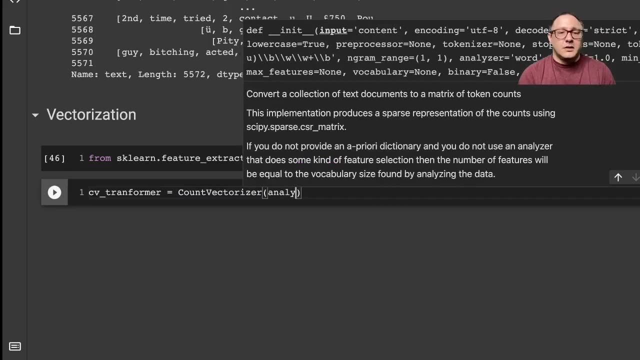 And that's how you're going to be counting them. So we'll initialize our count vectorizer And you know what I may say: cvTransformer for count vectorizer. The analyzer we're actually going to use in here is going to be our own. 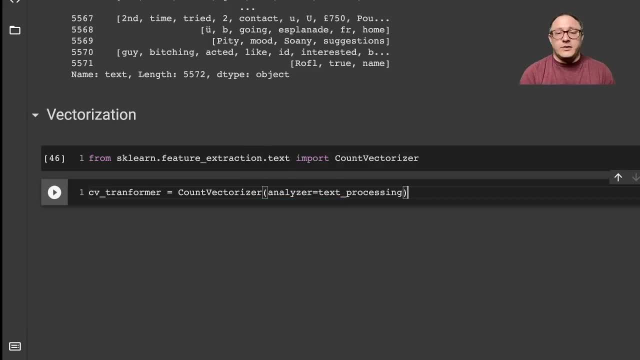 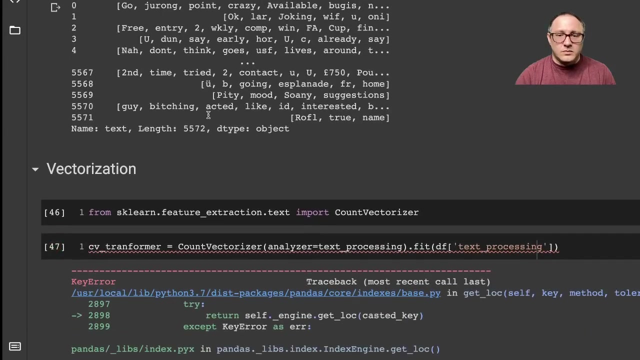 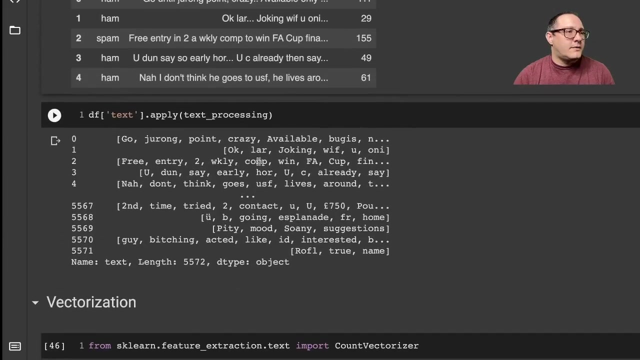 our text preprocessing- And again you can use some of the built-ins as well- Then we're going to fit this on our data frame And we want our text. So, oops, why did it not like my preprocessing? Let's take a look here. 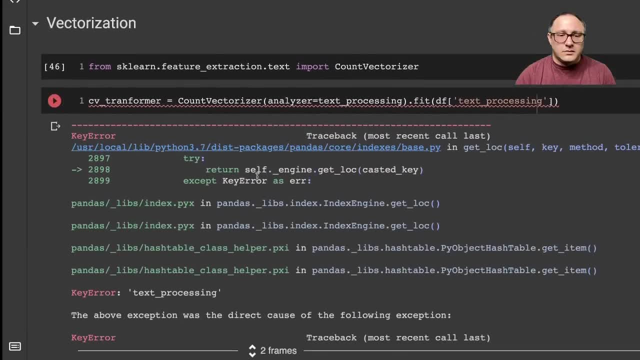 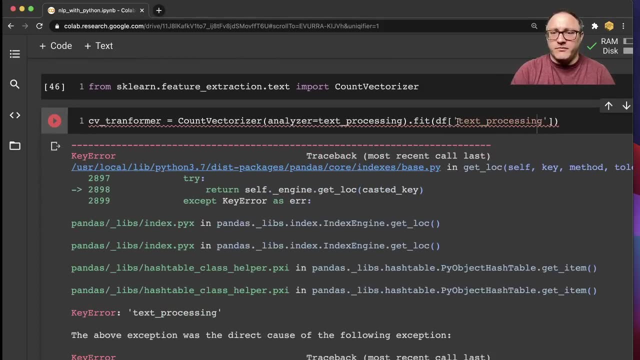 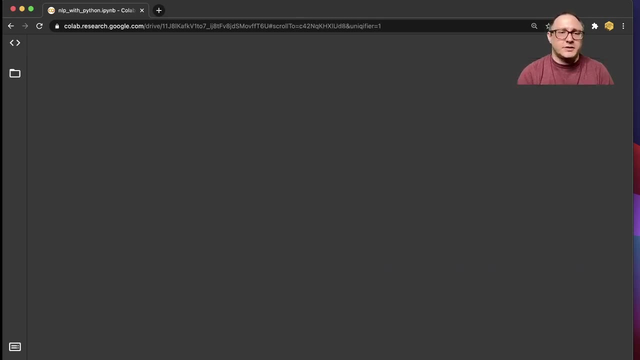 Hold on just one second. Let me see what happened. Whoops, So I was being a little silly here. I wound up filling in this instead of text. I actually wound up filling it with text preprocessing, thinking about our preprocessor. So 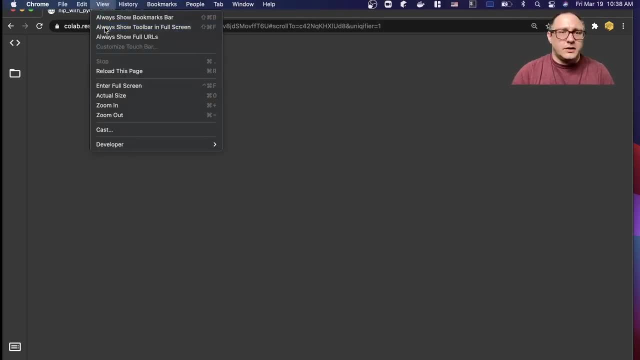 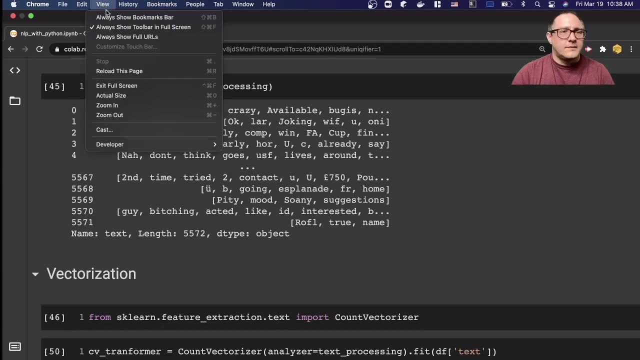 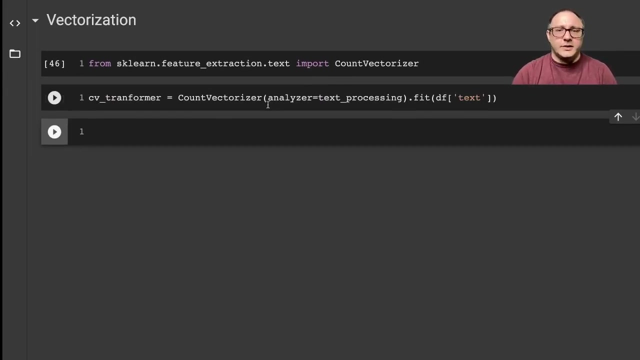 Okay, So let's go on and, oops, let that run for a second while I fix this In here, All right, And so let's actually take a look at now. notice, we did this in two ways. We actually initialized our and did our fit in one. 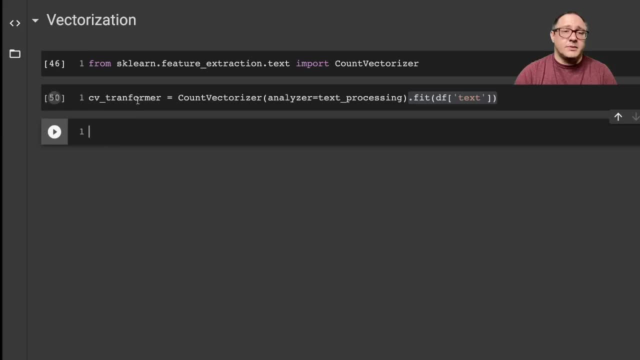 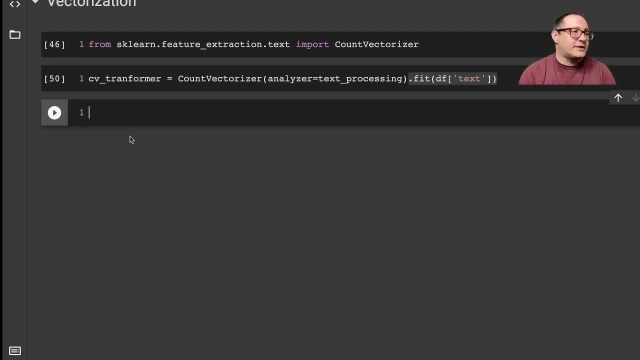 Okay, Some people like to do them in two stands, but that's okay, We can just do it all in one. So let's actually take a look at this. Let's take a look at how big our vocabulary actually is now. So, print, I don't actually need that. we need the length of our CV. transformer, dot and 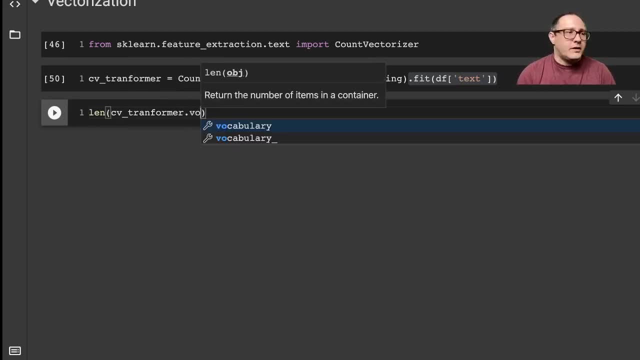 here we want our vocabulary and grab the vocabulary with an underscore, And so here you can see that this is actually pretty big. We have 11,425 words, And then so let's actually go on and take a look at, For example, what would happen with some of our messages, and look at what would happen. 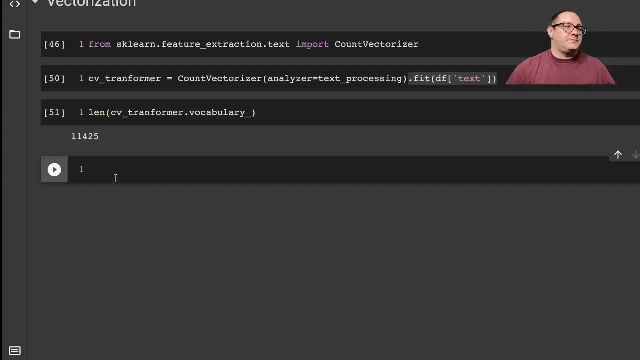 if we transformed maybe a specific line for our bag of words. So let's go through and see about what do we want? Text one, So we'll still grab, I'll say text zero, because we grabbed that first text message to look at it before. 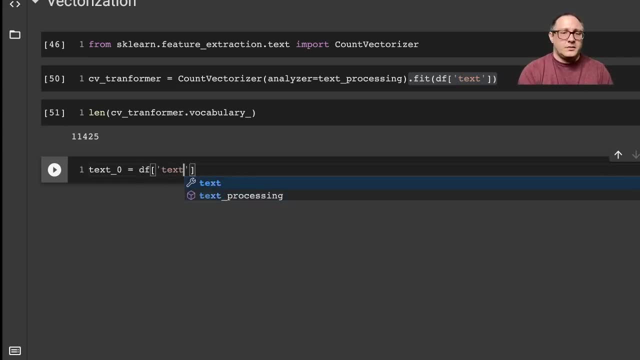 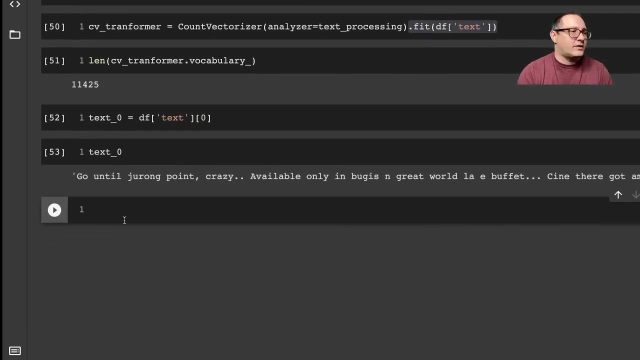 But let's do df text and we want zero, So text, zero. this is that. go until blah, blah, blah. And so then let's actually use that count vectorizer to transform the data And let's do- we'll call this our bag of words- zero, zero here. 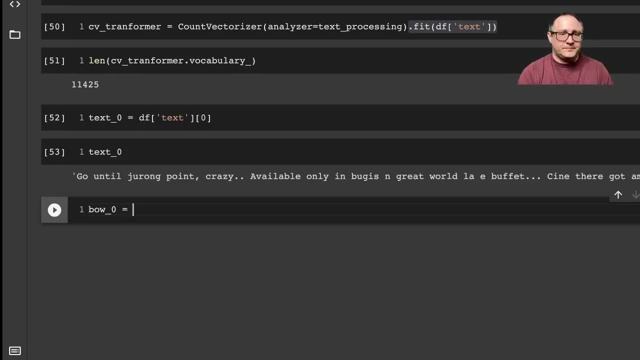 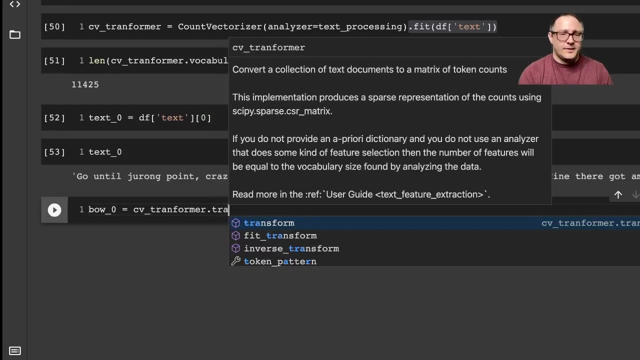 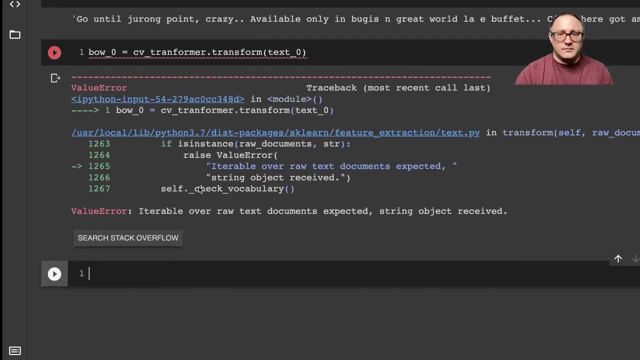 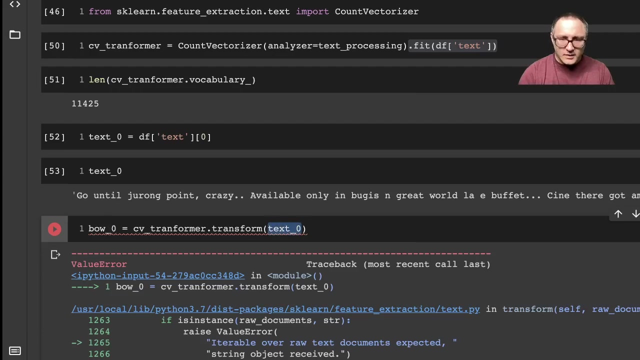 Okay. And then we want our CV transformer here and we want to throw in. we want to throw in our text: zero, Oh, whoops, And we need to put this. this actually needs to be in a list because again it has it. 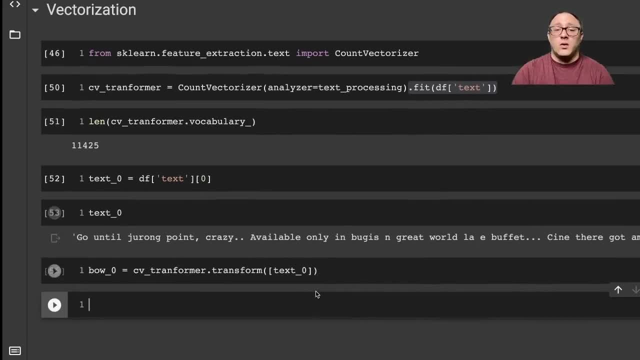 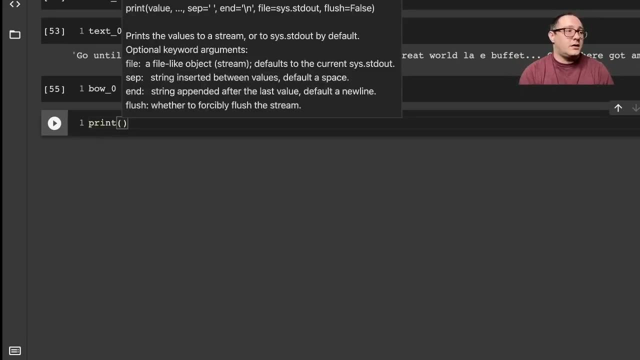 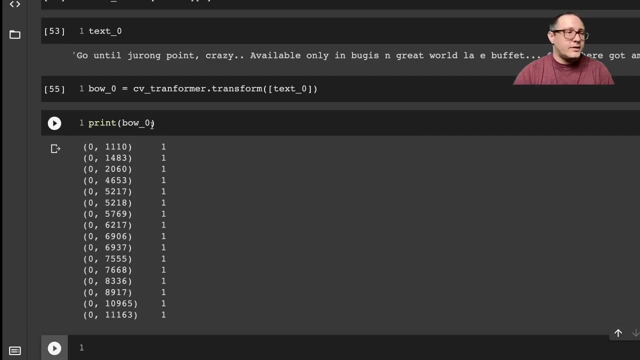 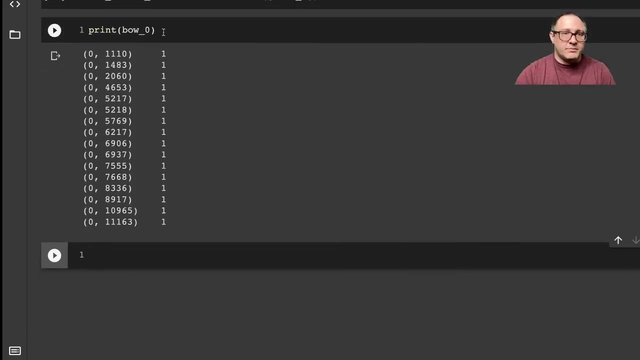 has this expectation that it's going to be drawing in a whole list. Okay, So let's do that. So let's take a look at what, what this actually looks like. So our bag of words: zero here, and let's also grab in. let's also grab in our shape. 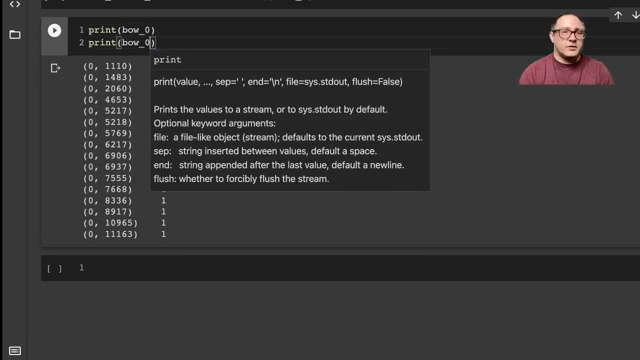 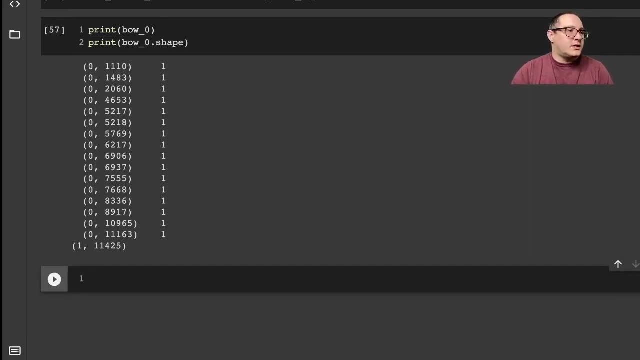 as well. So let me go in and print bag of words: zero dot shape. Okay, And so what this is going to go is that there are going to be how many unique words here? 1, 2,, 3,, 4,, 5,, 6,, 7,, 8,, 9,, 10,, 11,, 12,, 13,, 14,, 15,, 16,, 16 unique words in this, in this. 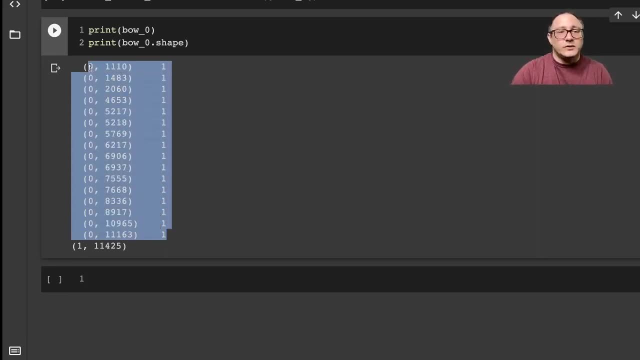 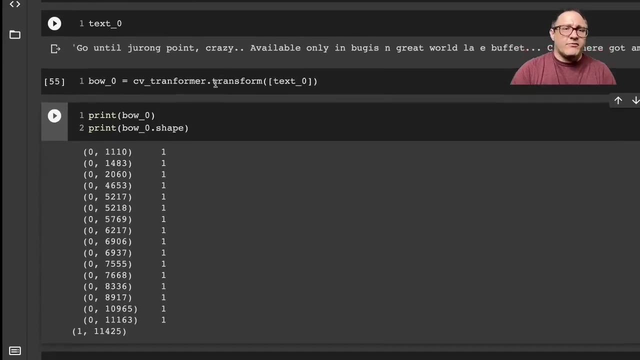 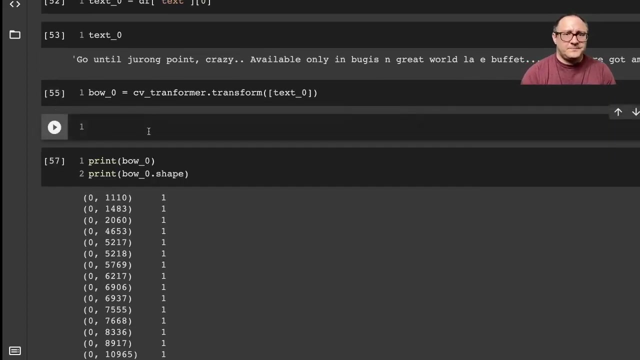 instance. Okay, So notice, all of them only appear once. Let me maybe, let's see. Okay, Okay, So let's grab. I want to grab another example where we have more than just ones. So this is actually very, very relatively unique. 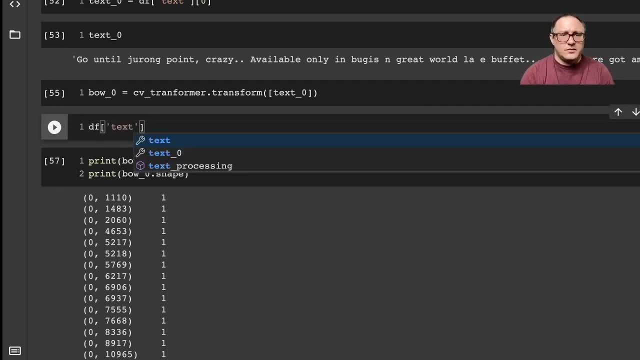 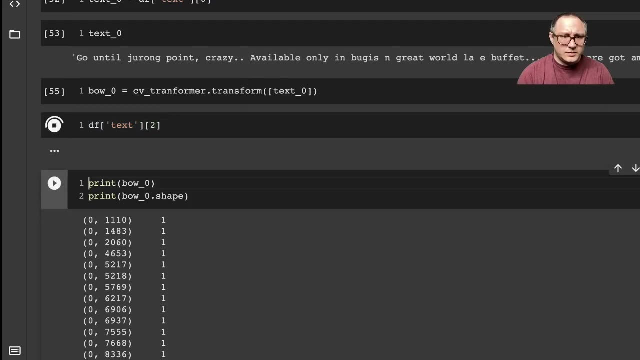 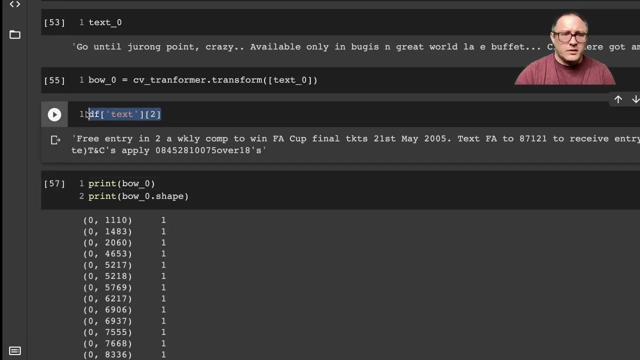 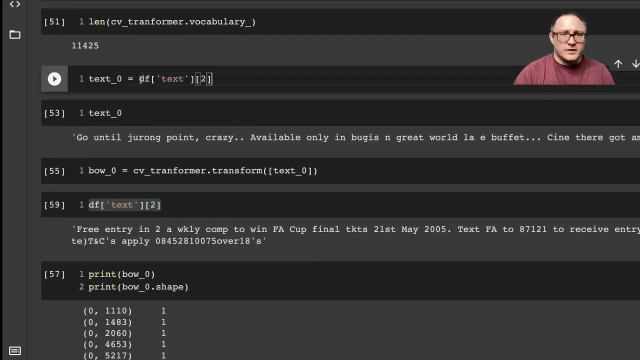 Let's look at, let's look at one. what was one? uh, two, Okay, Okay, Okay. So I'm going to go on and put: I'm just going to overwrite this, I know, I know it's it's frowned upon, but it'll be fine right now. 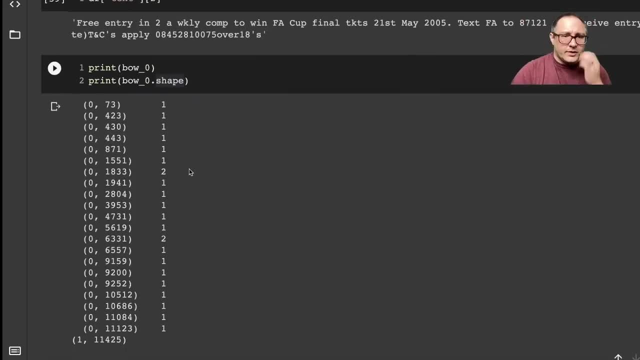 Um, and so here you can actually see that there are um again. there's probably 20 unique words here, but there are two instances where there are multiple counts of a of a word. Okay, Again, this is. this is. this is just an example. uh, to see. 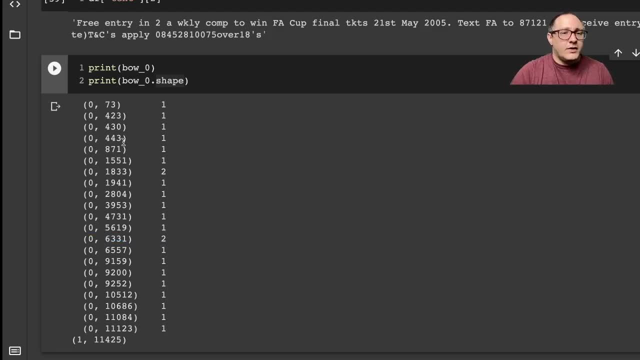 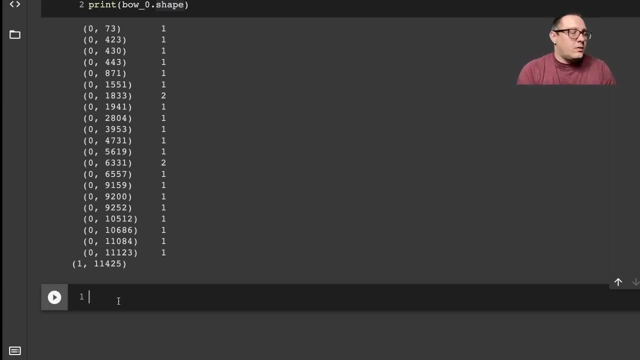 Um, so we can actually go through and, for example, we want to see these words that were mentioned twice: Okay, So we can grab that little uh codec here, that index, And so we can go and do something like: um, we want to see what our CV transformer we 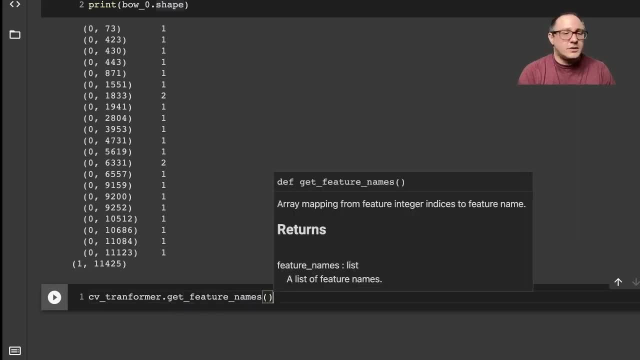 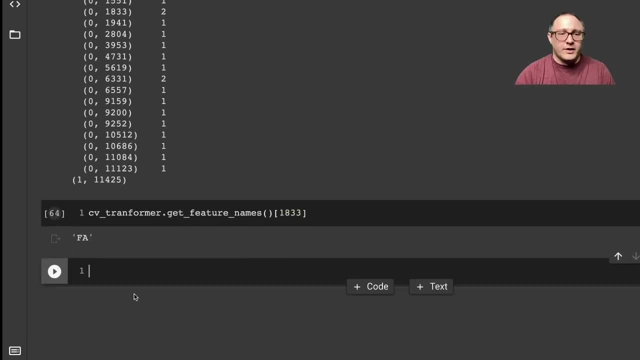 want to uh get feature names and then we can actually just put this: oops, we want to put this in to do our bracket notation, And so that one was FA again. I don't, I don't know what FA cup final. 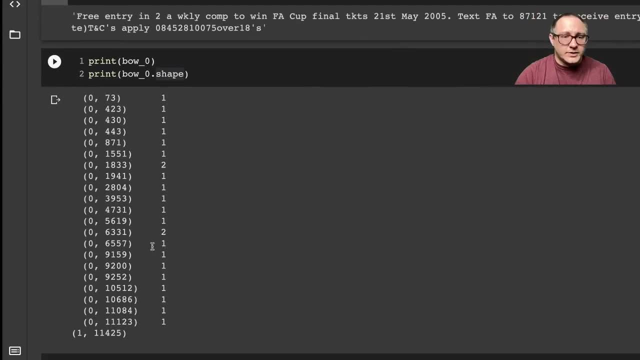 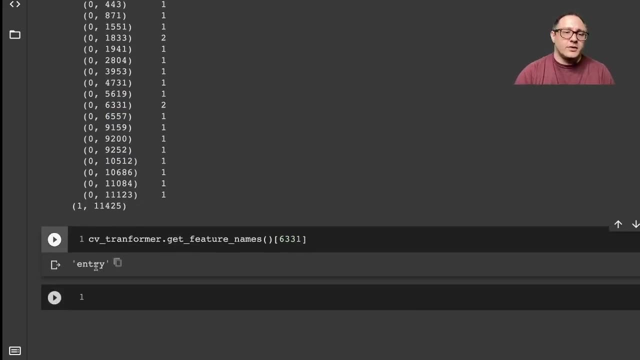 So maybe some sort of soccer world cup? Uh, and what's the other one that had two? so 6,331 entry. So again, maybe they're looking for entries into some world cup. So that's a very interesting way to check that out. 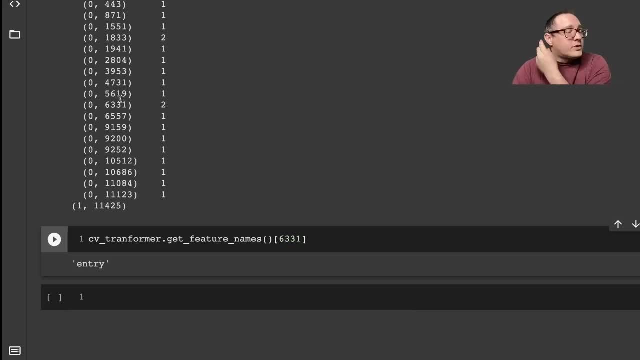 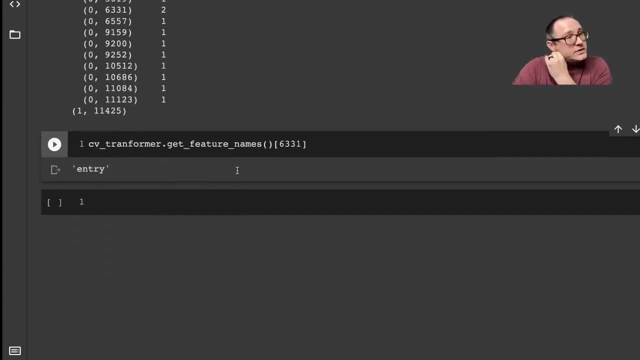 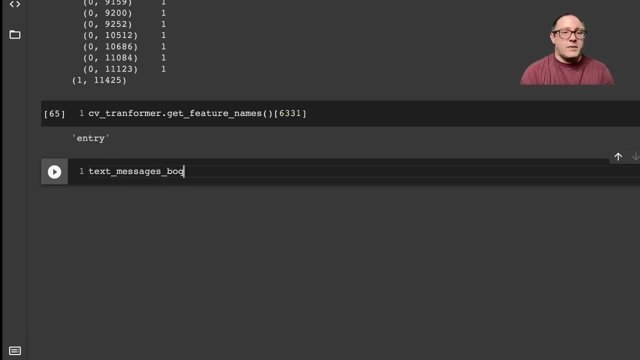 Now, Another thing that we can do is we can use our transform object for our this bag of words, Okay, Uh, on the entire dataset. So let's, let's go in and actually do that. So let's do a text messages, a bag of words, here, and we'll do our count. vector transform. 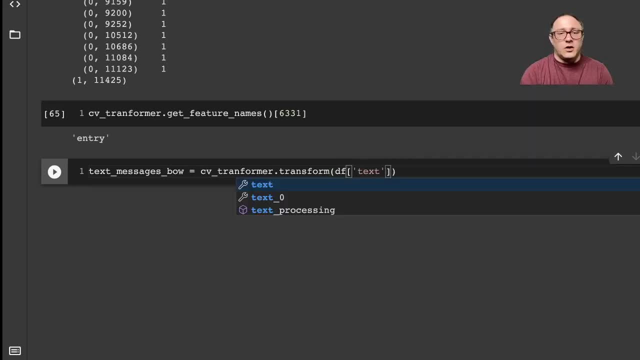 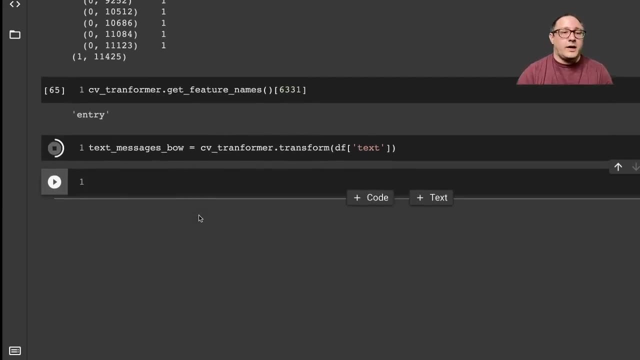 on it And we are going to do this on all of the words. So again, this is this. again may take a little bit of time, So I'm going to go on and we'll look at creating up a piece of code here that we'll take a. 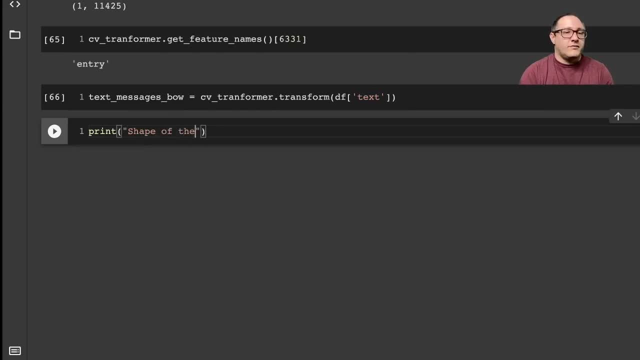 look at it. So we want the shape of the sparse matrix in here. Uh, and this one. I want this to be an F string and we're going to do our um text messages. bag of words, dot shape. Okay, 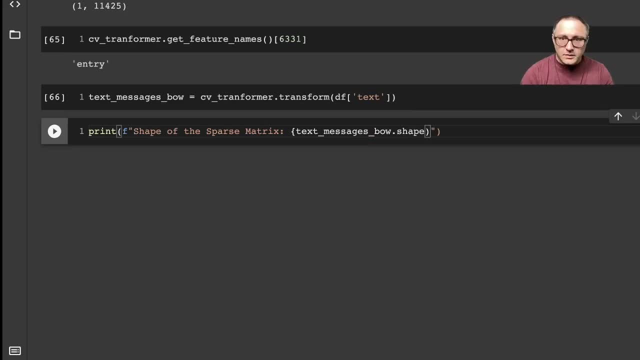 Oops, And we also will do something like print F string here: uh, amount of non zero occurrences, Uh, and so what? what this means here is that it'll actually count out how many times that there was a non-zero component. So we have, uh, where there's an actual word that's available to us, uh, and we'll do here. 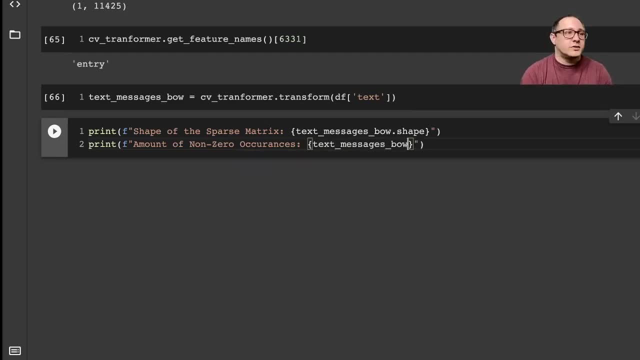 is Text messages bag of words dot NNZ. So that means for uh our uh non-zero instances. So again here we see that our sparse matrix is uh uh 5,572, uh long by uh uh 11,425. 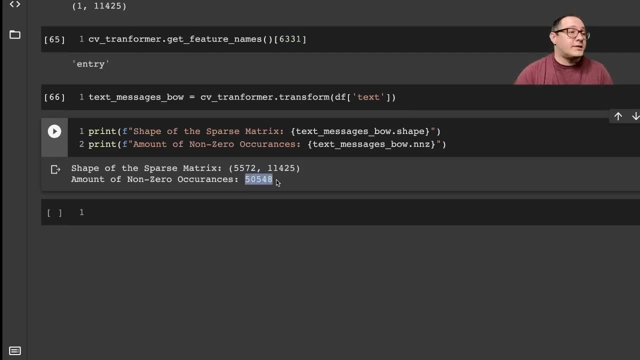 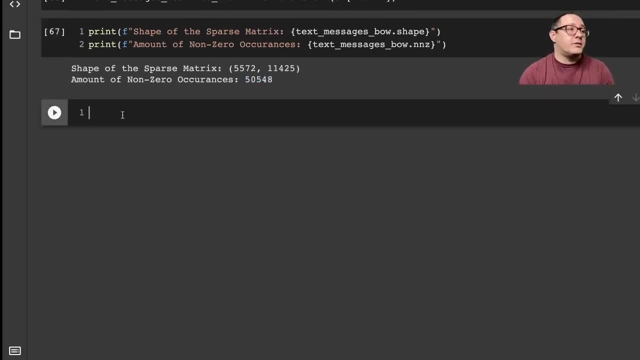 wide. We have 50,548, uh, non-zero, um occurrences, So we can also go through And measure up here the sparsity. So let's do something um like again, so sparsity. let me actually go through and actually. 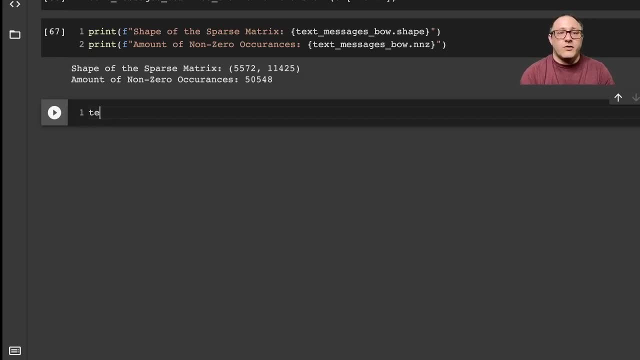 do this. So, um, uh, messages, not messages. We have our text messages bag of words and we want our uh dot NNZ. Okay, So our non-zero occurrences divided out by our messages, Oh, Okay. 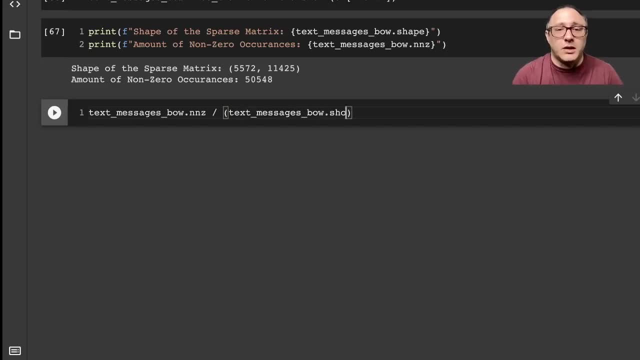 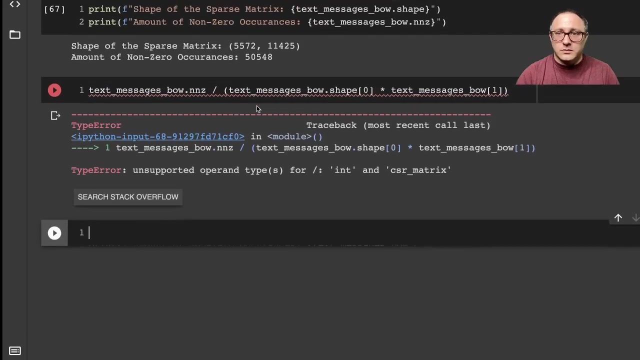 So we have our text messages shapes, Okay, And so it's going to be the shapes multiplied by each other, So how many observations we actually have? And so this is multiplied by zero, And then we also have our text messages shape. here um one multi, uh, whoops. 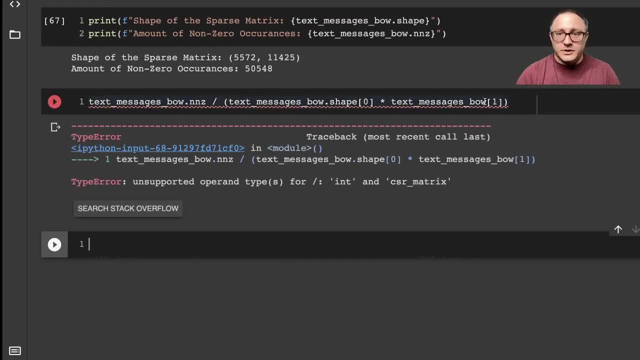 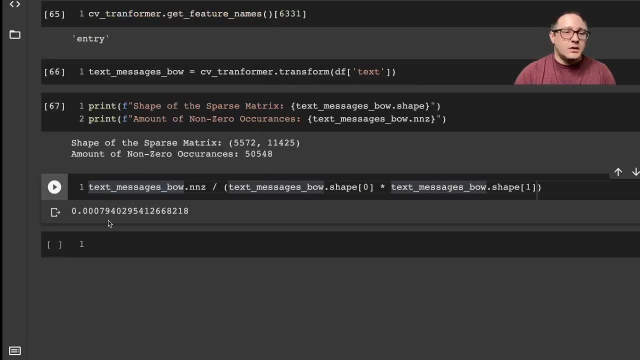 What didn't it like? oh, whoops, here, dot shape. Okay. So okay, And I need to multiply this out, cause this is actually really small, but the sparsity of this is basically zero, Okay. So, even if we multiplied this out by 100, um, I'm going to name label this sparsity. 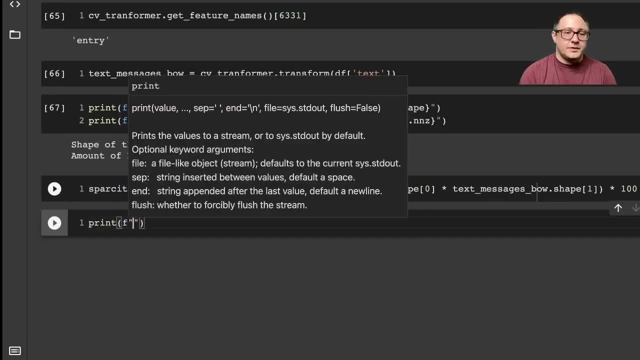 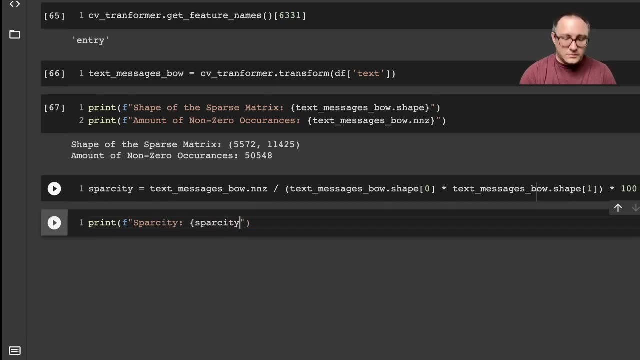 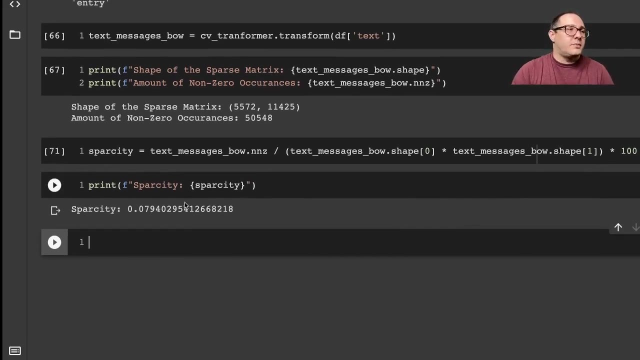 And so then you could do something like um print, uh, Okay, So this would be our sparsity. um, again, it's uh close to zero, but not quite Um, so we also need to probably take into consideration again. 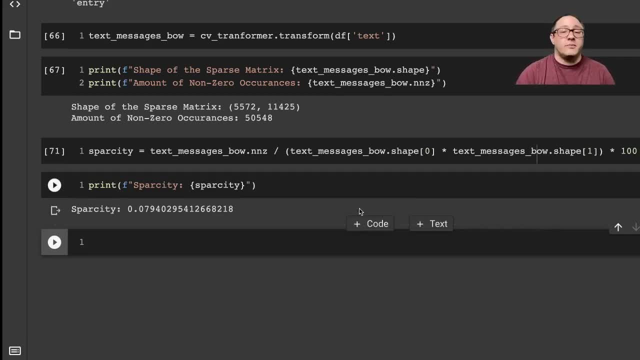 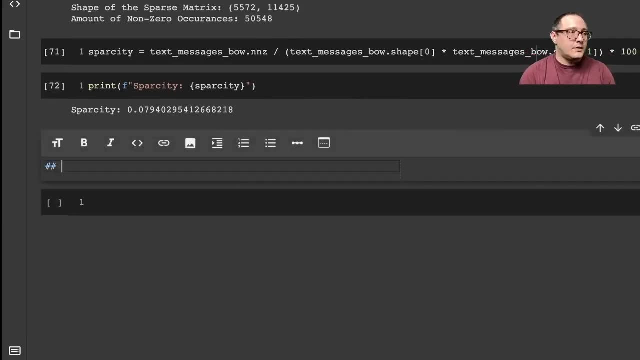 So we've done some normalizing, that type of stuff. What's going to be next for us is going to be our firm, um, our term, frequency, inverse document, uh, frequency, So our TF, IDF, Oh Okay. So this is actually um very important for us and and what we're going to be uh doing. 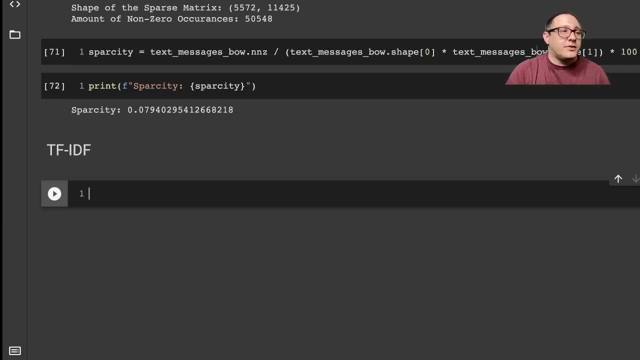 a lot of the time. So let's actually do this and talk about this in a way. So consider, we have something that has like um a hundred words, where the word um, Apple is going to appear maybe three times. Okay, 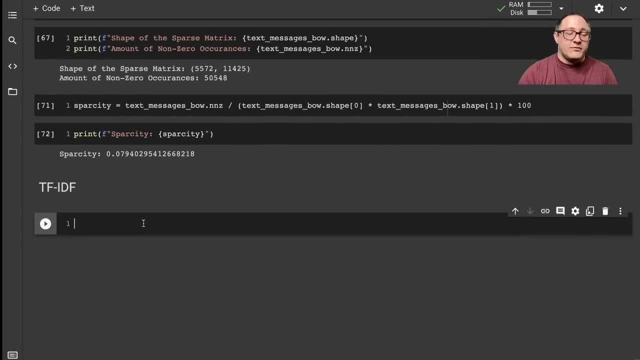 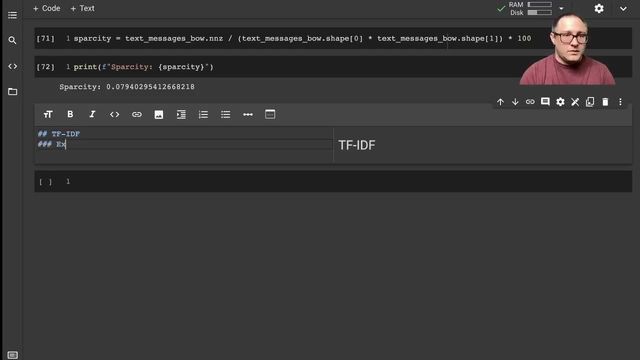 Well then, the term frequency of of that. Okay. So if we have- uh, let me actually write this out here- Okay, So example, Okay. So, for example, um, we have 100 words, okay, And we have, um, I don't know, maybe actually let's do this as a banking example. 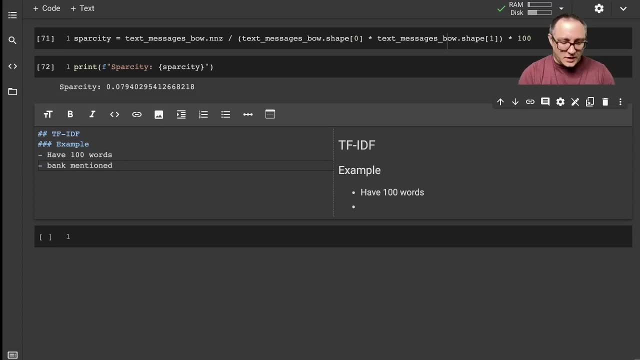 So maybe the word bank is mentioned, uh, five times. Okay, Now the, since it's mentioned five times, the term frequency, okay, is going to be our five divided by 100.. Okay, And then, and so let's, um, let's do this as a 0.05.. 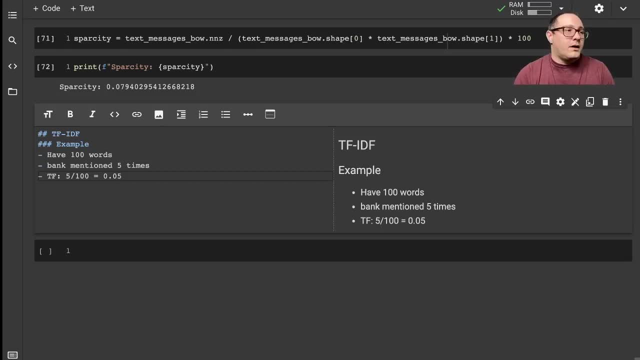 Now, if we assume, for example, that we have maybe, um, I don't know, a million, uh, or maybe even a hundred million documents, okay, or 10 million documents, It doesn't matter. Uh. and with the word that appears, maybe, uh, with the word bank. 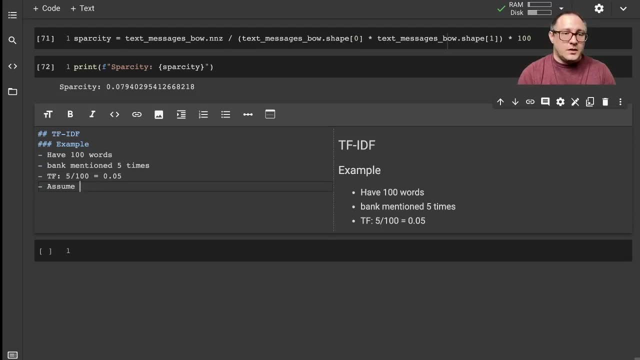 So let's say assume, okay, Uh, 1 million capital, M uh documents, okay, And um, so in the, the word in there, okay, So bank appears. uh, let's say we have it as, uh, I don't know a thousand times. 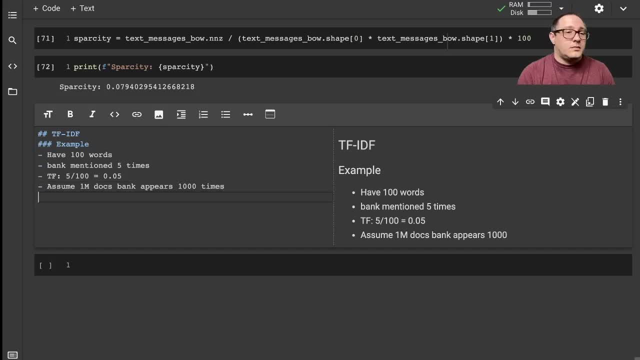 Okay, So Okay, Uh, what are we going to do with this? Well, we need to also have the inverse document frequency in here, and that would be, um, here is log of that: 1 million, okay, Divided by that 1000 times. 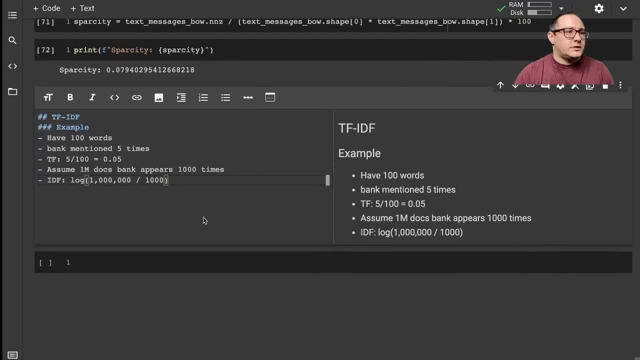 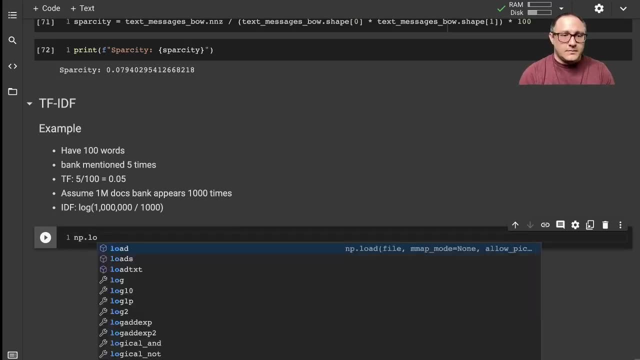 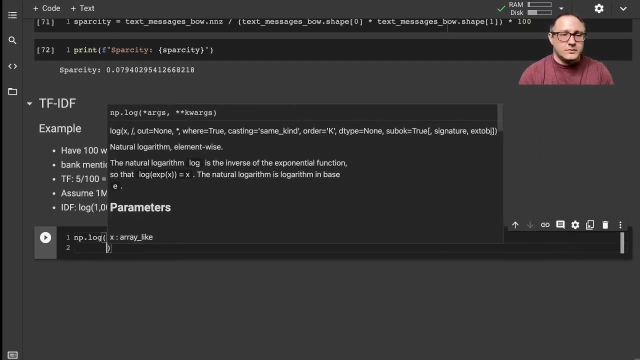 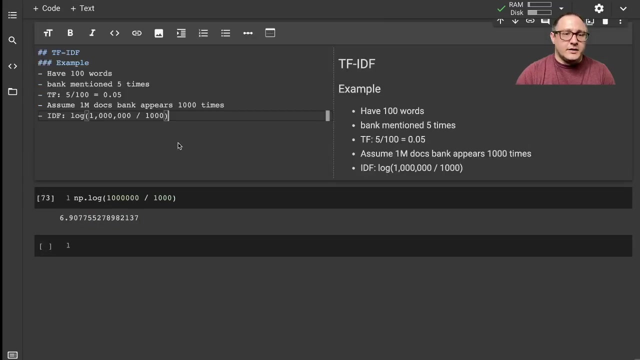 Okay, Uh, and so actually let's, let's maybe see what that would be here real quick. Um so MP dot log here and we have million divided by 1000 in here, And so that's a six point. So let's say it's going to approximate approximately, going to be, uh, seven. 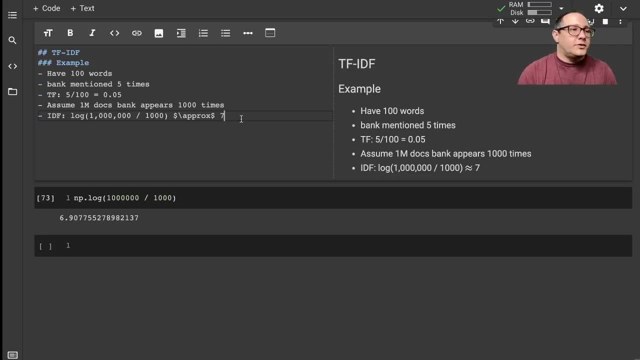 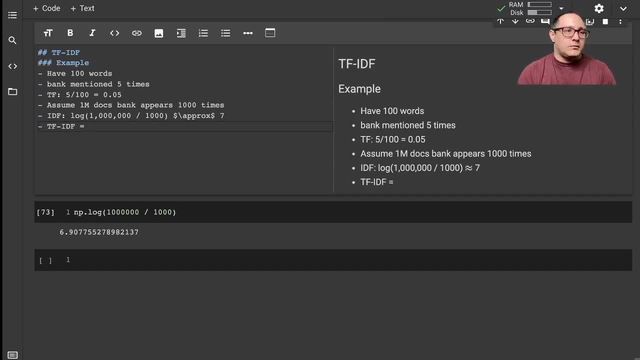 Okay, So what we actually would do here is for to calculate our TF IDF. okay, That would be, uh, our term frequency, uh, multiplied by our IDF. So we can actually, we can actually do that in here. So multiplied by 0.05.. 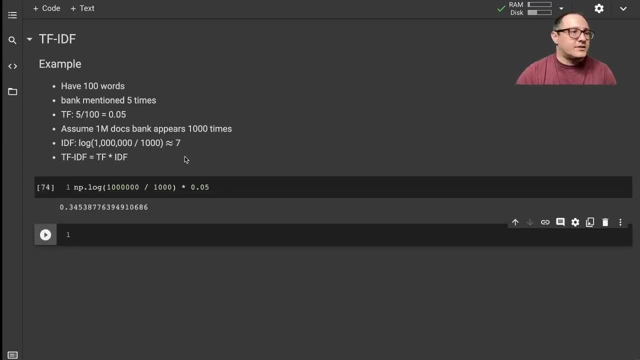 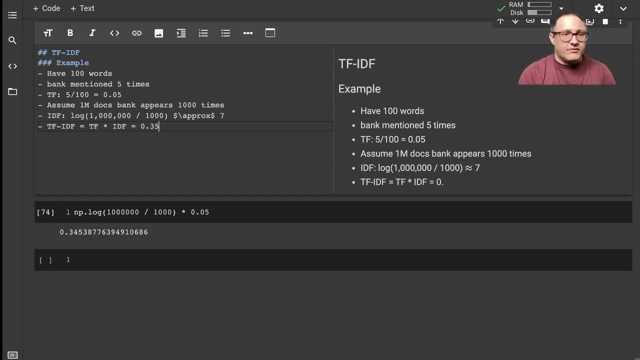 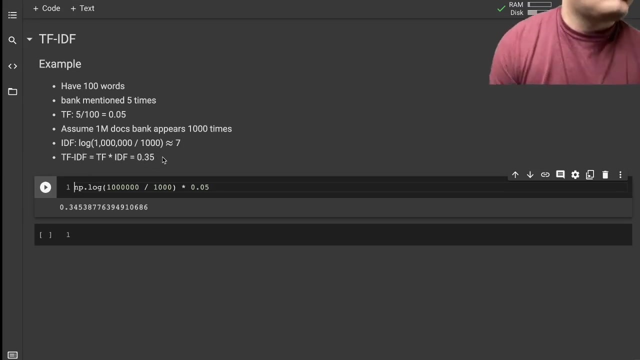 Okay, And that'll give us a point as equal to 0.5.. Okay, Okay, Okay, Let's just say three, five. So this is our inverse, uh, document frequency, And so this is. this is actually telling us um some words, okay. 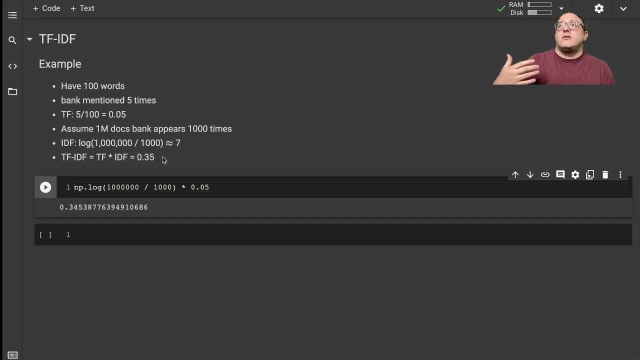 Aren't going to be as important because, again, if it's, if it's, if it physically manifests a lot in a document, it's not necessarily going to be, it's not going to have a lot of information in it. Now it may, may be the topic itself. 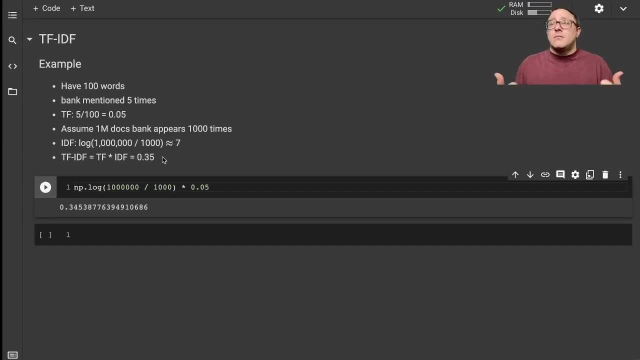 Okay, So the term frequency is important to tell us, maybe, the topic, but when we talk about the important words that are unique to the dataset, That's where we need to calculate up this inverse document frequency to help kind of weed out those very common words. 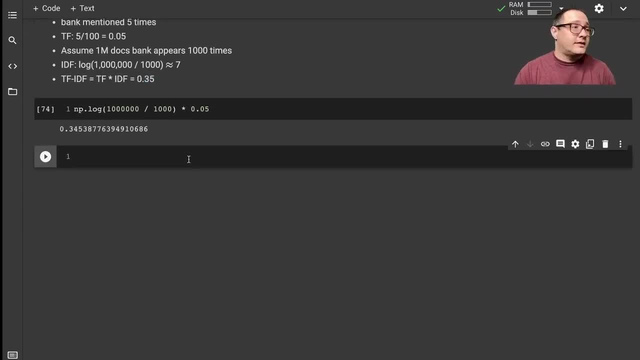 So let's go on and use scikit-learn to actually um calculate this up for our dataset. So from sklearnfeatureextractiontxt we want to import the TF IDF transformer, So let's do, uh, TF IDF. Okay. 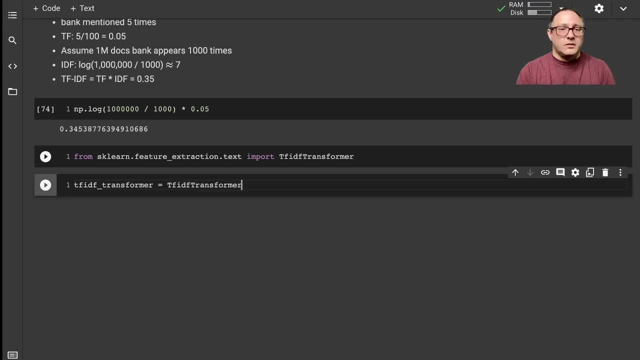 Transformer in here, uh, and we're just going to fit this on our data, um, and which one are we going to do this on? Let's do this on our bag of words already, Uh, and then let's actually take a look at um. we need to transform this, uh, for a specific. 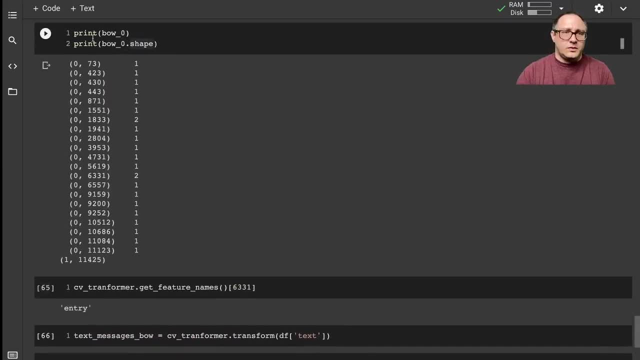 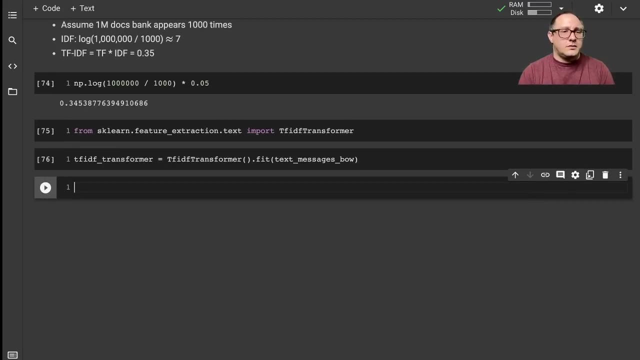 one I think I used um- Oh, it was a bow zero, All right, So let's do um. TF IDF zero is going to be equal to our TF IDF transformer transform, And we want that on our bow zero. 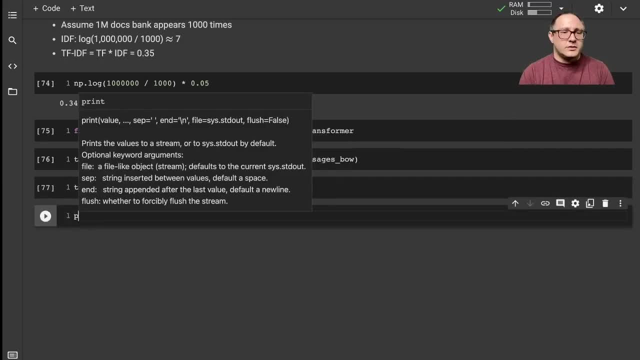 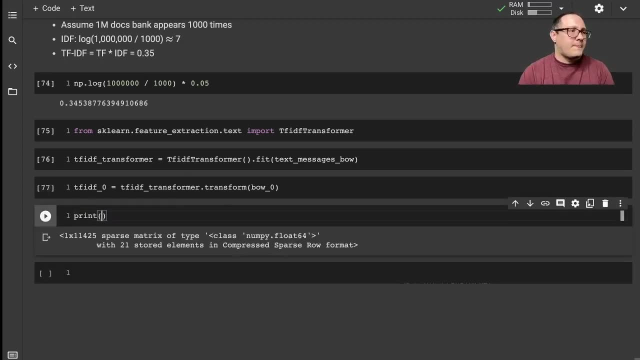 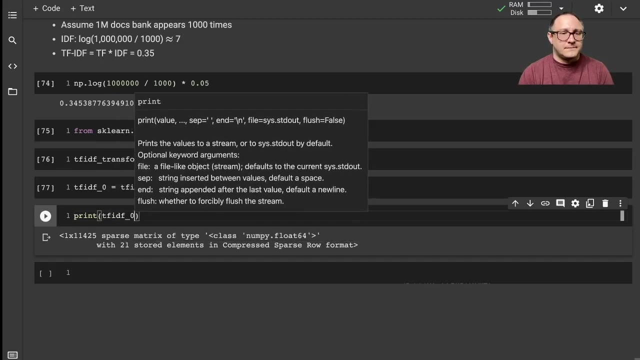 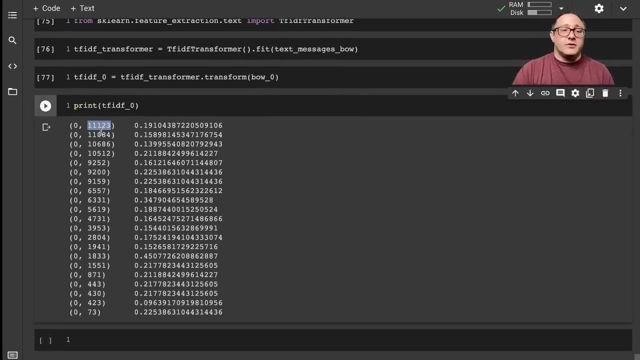 So what we had before. So let's take a look at the TF IDF. Okay, Okay, TF IDF- zero Whoops, There we go. So you can see here that now we have the inverse document frequency for each of those words for this particular text message. 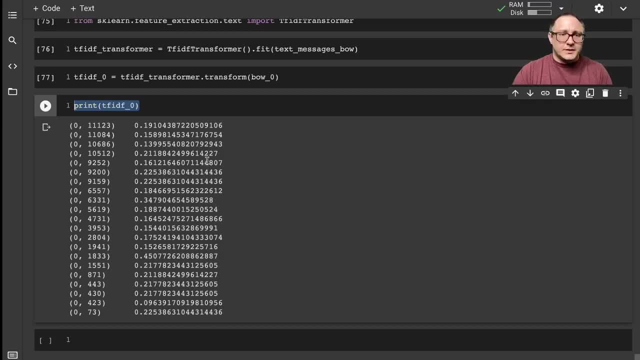 So, um, let's see What are some of the high numbers in here. Let's see, Okay, So this one and again- this is for the entire document- how it will compare for the entire document again. So here we have a really high number in here. 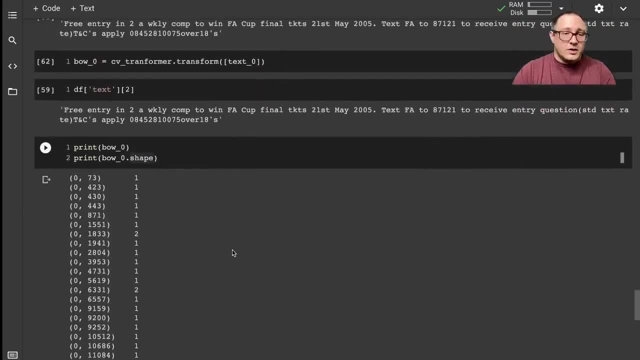 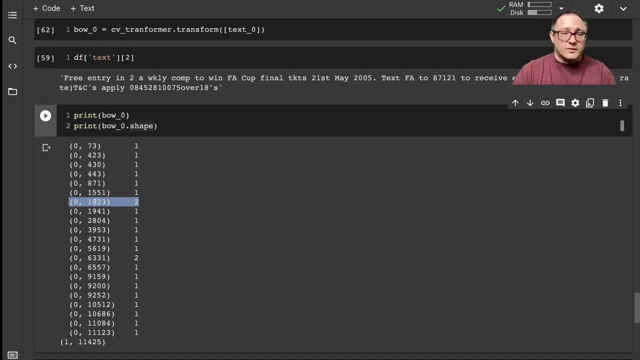 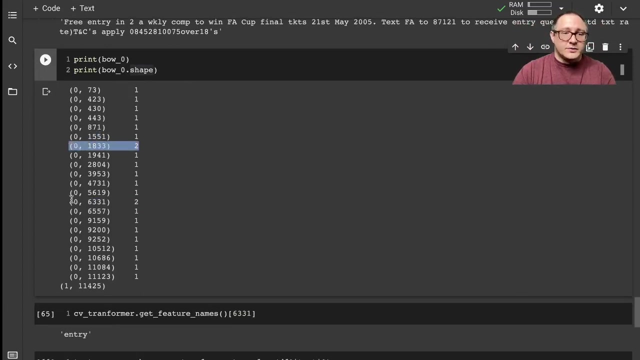 All right, Remember, um. go back to here. We see that the term for week frequencies here this was high, Okay, This one was high and this one was high, Okay, And I think this one was uh, this one was F a and this one was entry. 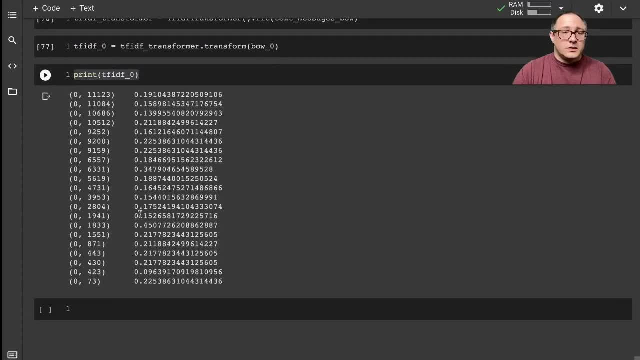 So then we would expect that those numbers are going to be high as well. Uh, So look here: this one's a 3.47, so 3.5, and this one here is has a high number as well. So those have a relatively high term frequency. 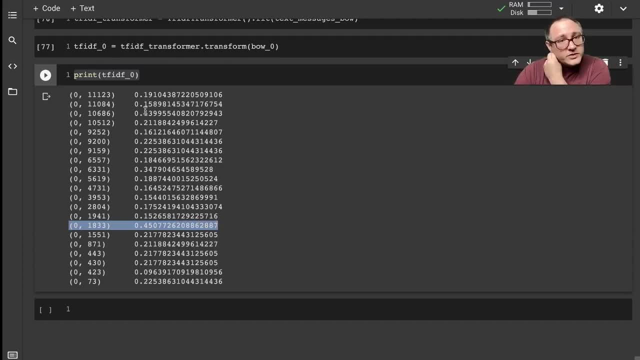 They're common. So then, if we look at the uncommon words, let's look for something with a zero. Okay, So this is. this is our zero. here is the lower level number, Uh, so let's look and see what this one is. 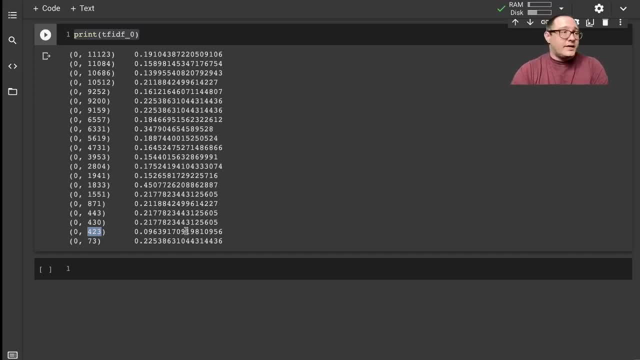 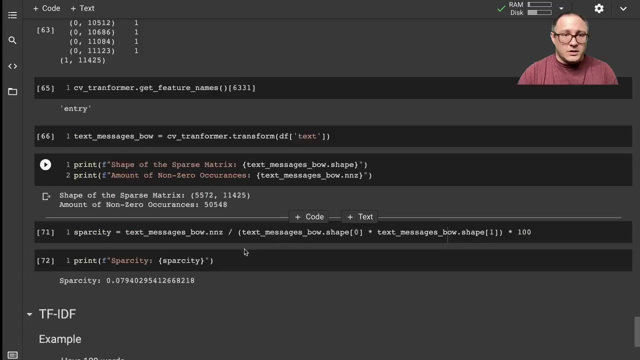 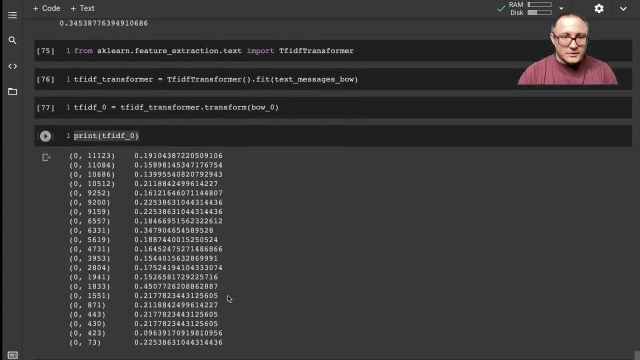 This, this one may have a lot of information, or it may actually be completely, um completely, useless to us. Uh, so let's actually go through and actually, uh, look at what that word is. I'm going to go and copy the code from up here really quickly so we can actually see. 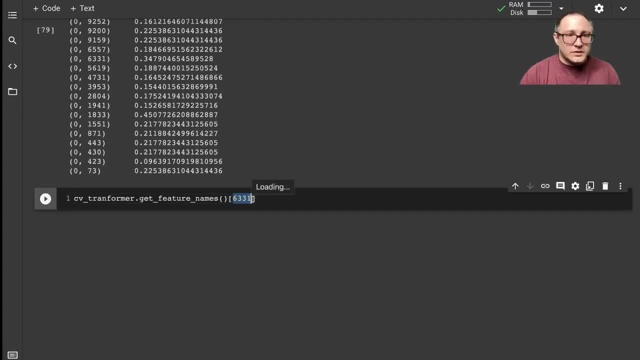 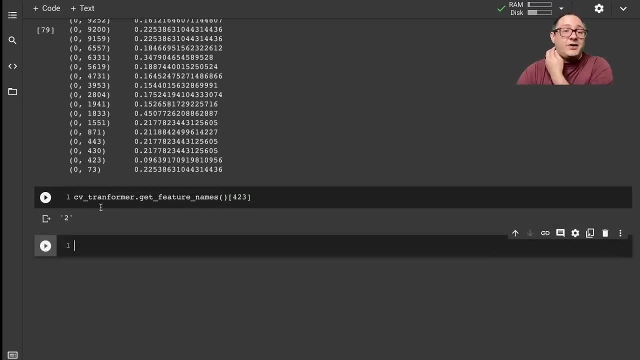 that word Uh, and it was uh 423.. Two, Okay, So it's actually. it's actually a number, It's a number. So again, maybe, maybe it's important that inside of this text, so maybe they're looking. 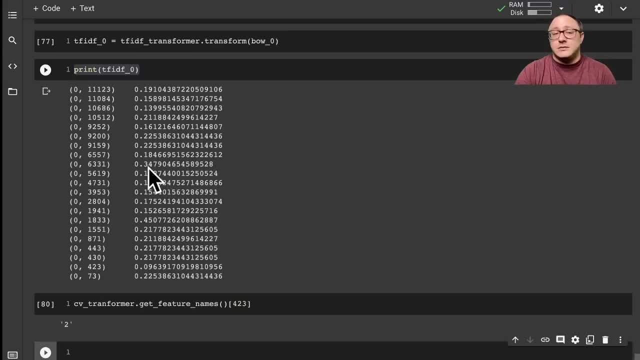 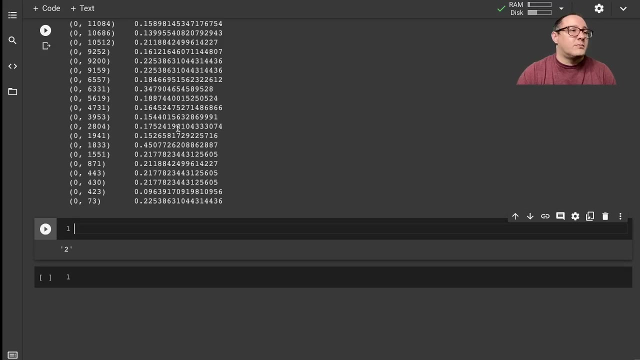 for two entries. Okay, Uh, for that, uh, for that FA, whatever the FA was, um, but again, that's, that's maybe necessarily taking it out of context. Um, so let's maybe look and go ahead and look at, for example, some of the term document. 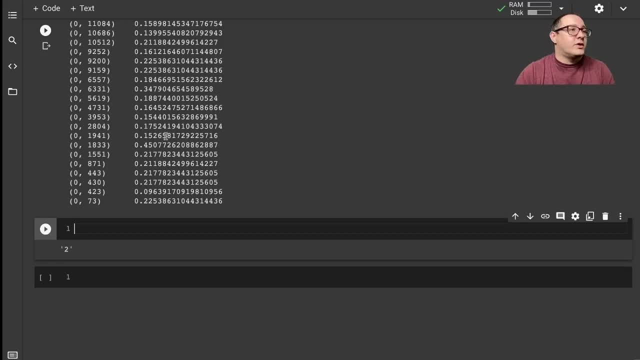 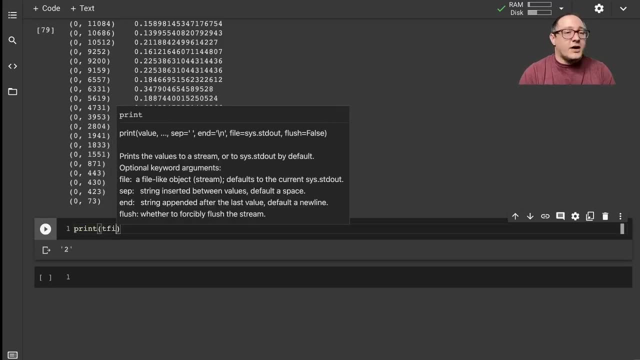 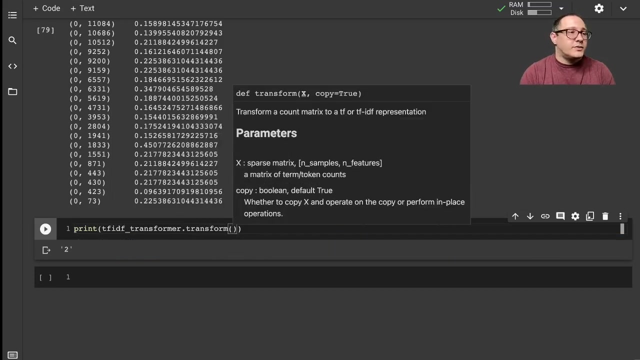 frequencies for some other words. If we want to, you can look them up by a specific word. Okay, What do you want? So let's do something like a print: uh, TF, IDF, our transformer, dot, transform here, And we're going to do this on our um. no, you know what we want. to check, uh, by a specific. 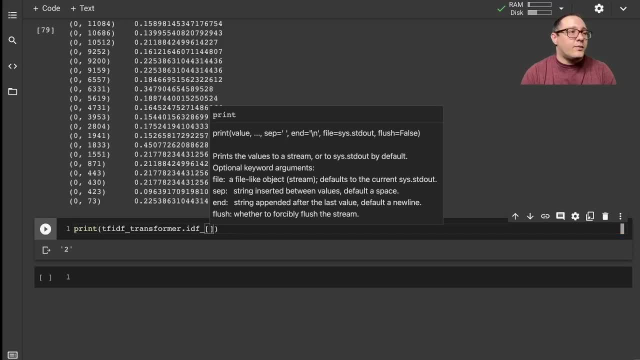 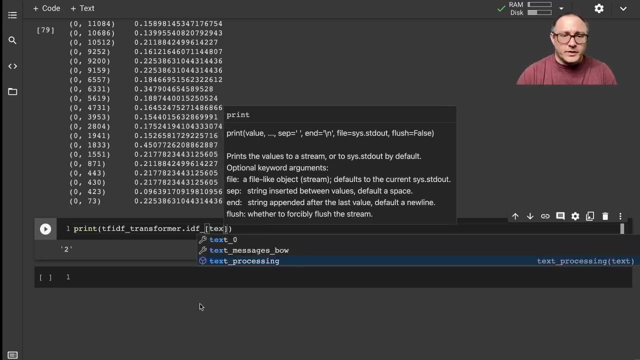 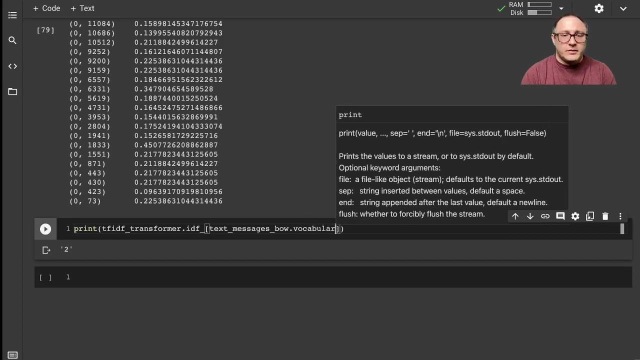 word. So we do IDF underscore here And then we do our, our bag of word. Oh, What was that? What was our vocabulary? Um, what did I call the? oh, there, it is. Text message. bag of words: uh, dot vocabulary underscore. uh, and we want this for let's. 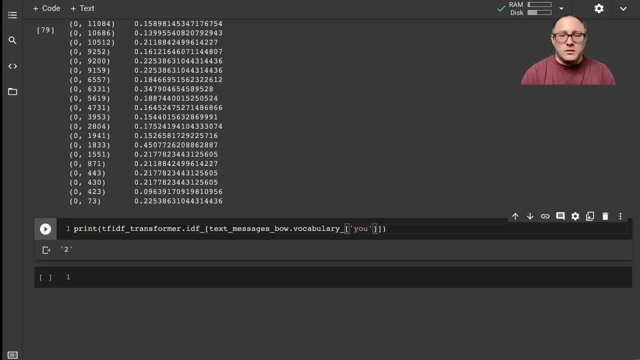 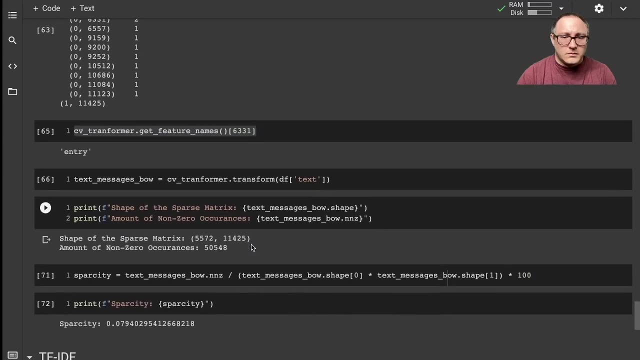 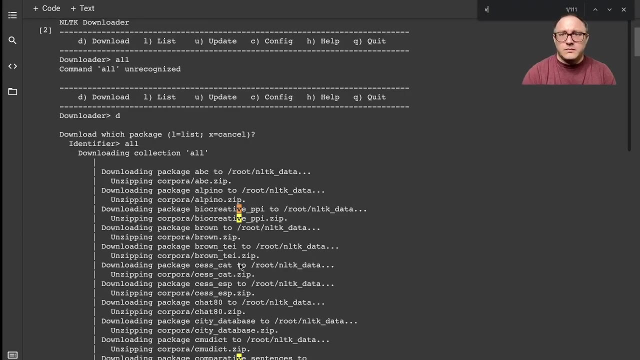 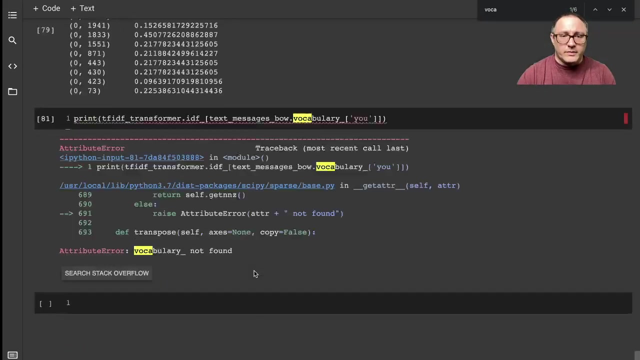 try um you. Okay, Okay, Okay, Okay, Where did? where did it go? Oh, okay, The transformer, See transformer vocabulary. All right, Sorry about that, I'm having trouble remembering what I actually wrote down. 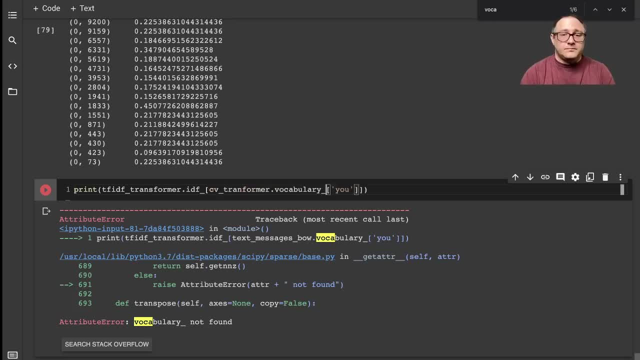 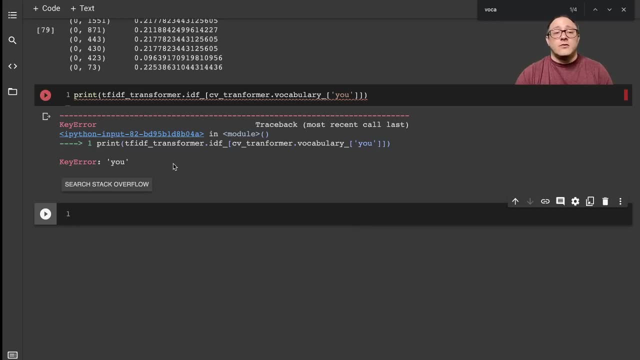 That's a problem, Isn't it All right? So you, oh can, Okay, Okay. So one thing that this won't work, for example, is going to be a stop word. okay, so it will not be in there, we will get. 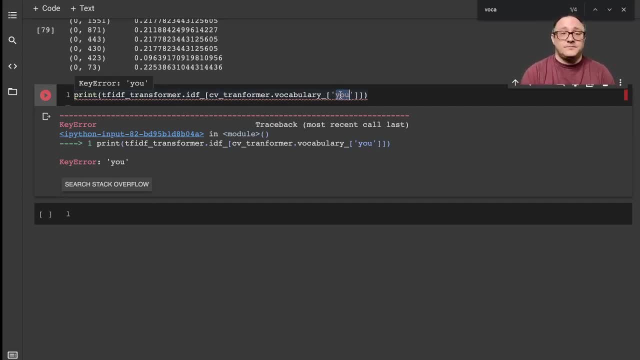 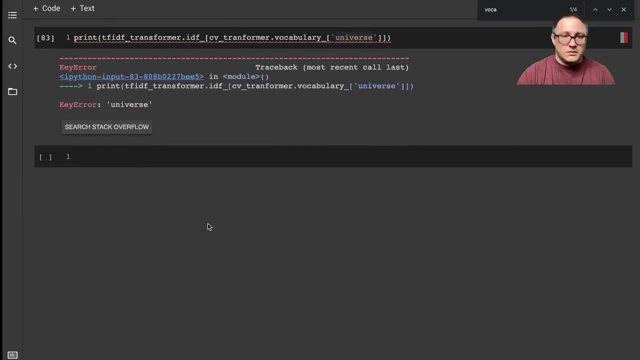 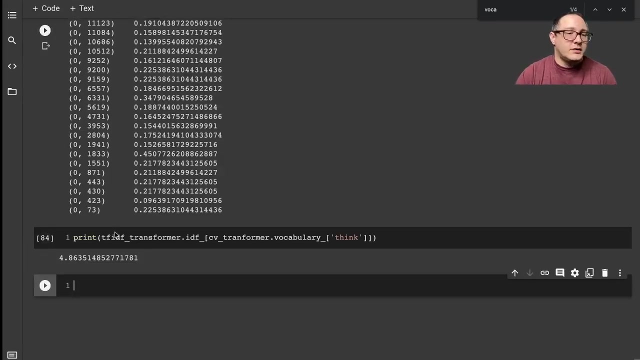 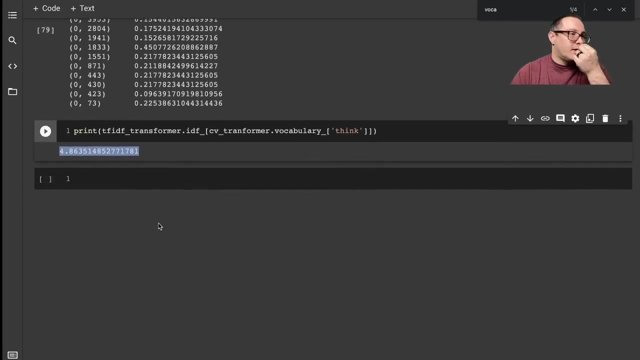 something uh weird. so let's try um universe, nothing, um, well, let's go up to a print here. uh, all right, let's do think: think okay. so this is the uh term frequency of think okay. so, uh, again, you can go on and you can look up words individually: um, and again we can always um, we can always convert the entire uh text. 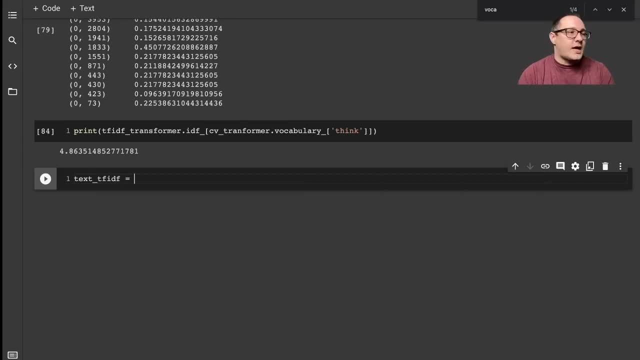 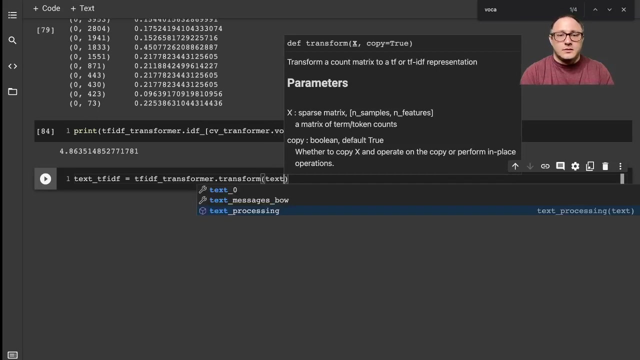 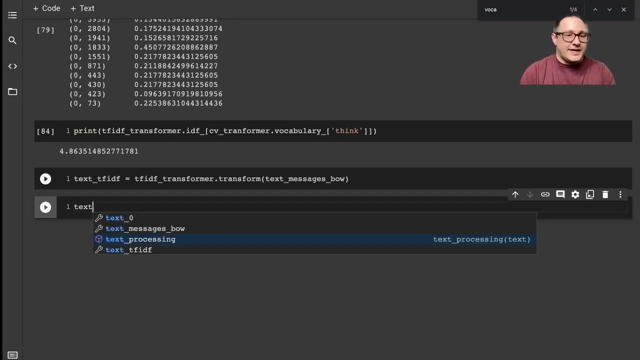 t, f, id, f, um, for the entire thing, for the entire data set, um. so we do the transformer, transform here, and we'll do this on our text messages for the whole thing, and then we can actually look at the shape real quick so you can see how big uh, this gets um. one thing is again: make sure that you have enough ram. 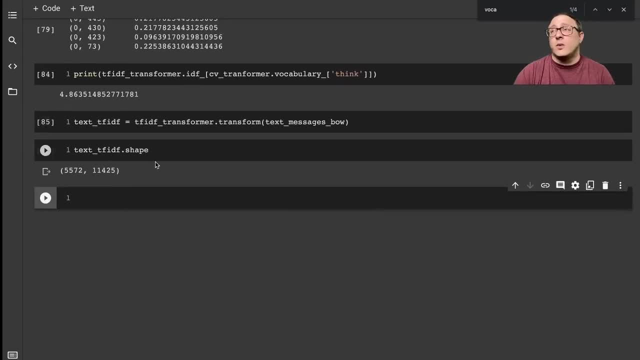 whenever you are starting to mess around with this stuff. again, this is just a toy data set of text messages. if you start looking at big documents or anything else, you're going to need a lot of text messages and you're going to need a lot of text messages and you're going to need a.